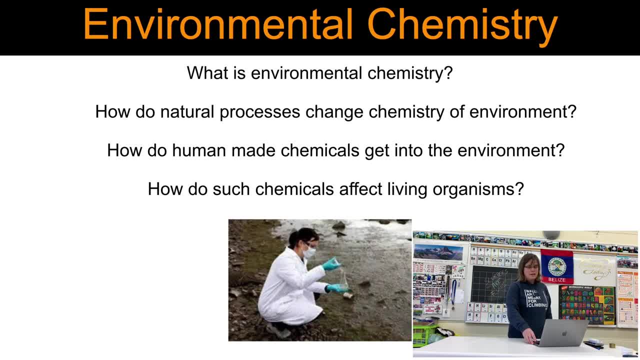 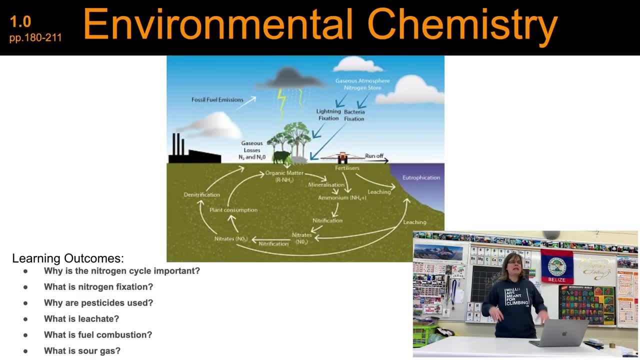 the environment, things like pesticides and stuff like that- and how do such chemicals affect the living organisms that are around us? So the deal is is that we're going to really be focusing in on a few things that are important, and you're actually going to see them in grade 10,, 11, and 12.. And one of the things that we're going to look at first is something called the nitrogen cycle, And the nitrogen cycle has to do with the amount of nitrogen that's in the air and how it becomes usable to us humans. This is a really important biological and environmental concept that 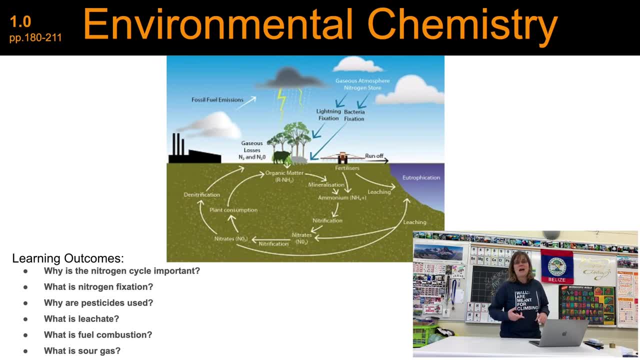 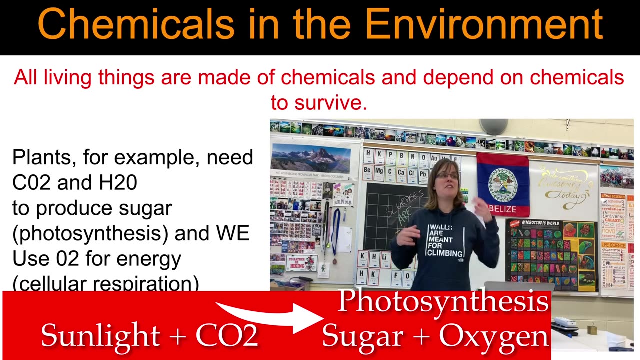 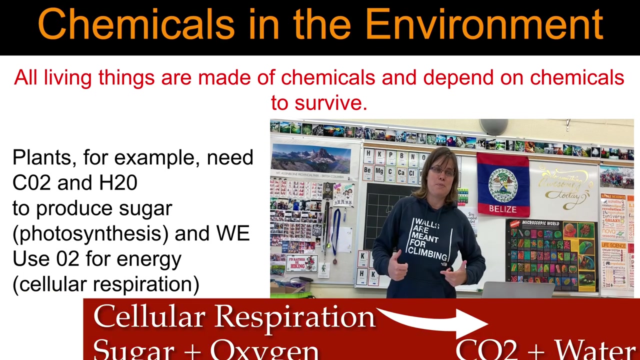 we need to kind of understand. We're going to look at other things like pesticides, garbage juice, fossil fuels that go into the environment and burn up the environment. So we need to understand those processes too. what types of gases are being released and what can we do about it. So here's the deal. you guys, we learned in grade 7 these two really important processes that are going to haunt you for life, And those two are photosynthesis and chemical respiration. The deal is is that photosynthesis is able to 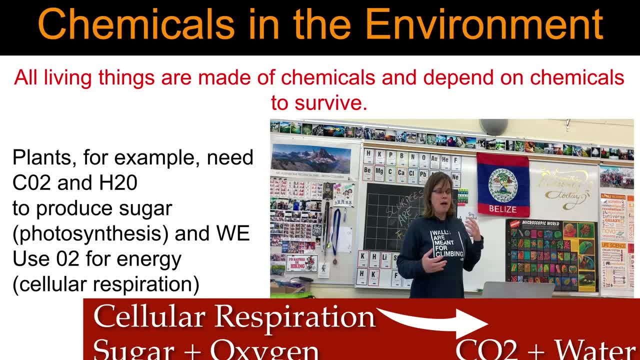 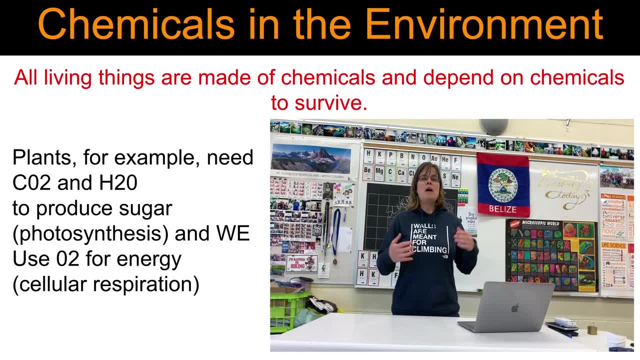 take in. they need CO2 and they need H2O to produce sugar, and then they also produce oxygen that we breathe, And so the deal is is that what plants take in is carbon dioxide. They drink that in and they need to drink. 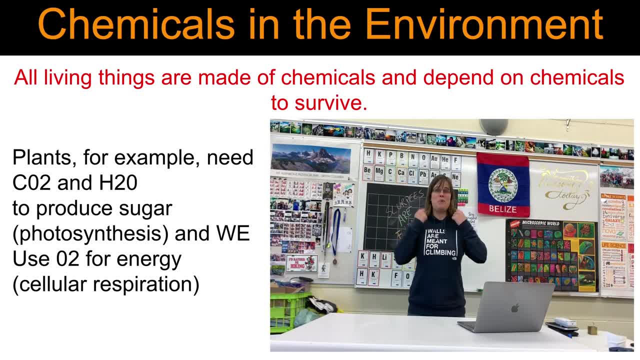 in water as well, to grow. They make energy, which is what we eat in salads, but they also make oxygen, And that oxygen comes back to us in a cycle called cellular respiration, because we actually breathe the oxygen that the plants give us and we are able then to be able to produce energy, and we're able 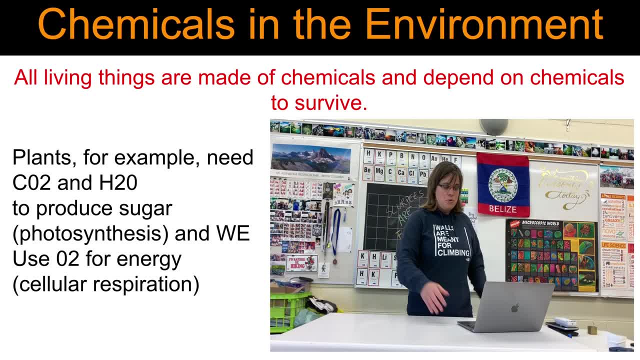 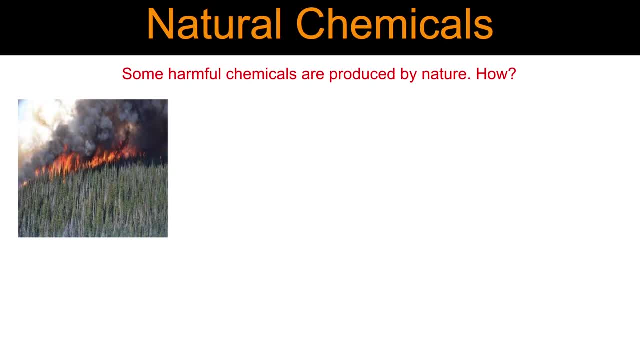 to do all those processes that are important for our lives. so those are important chemicals and those are important processes in in our environment. so some natural chemicals, so some harmful chemicals, are produced by nature. so you need to understand that gases, all gases, are not safe. so, uh, right here we have a forest fire and the forest fire is producing at this time. 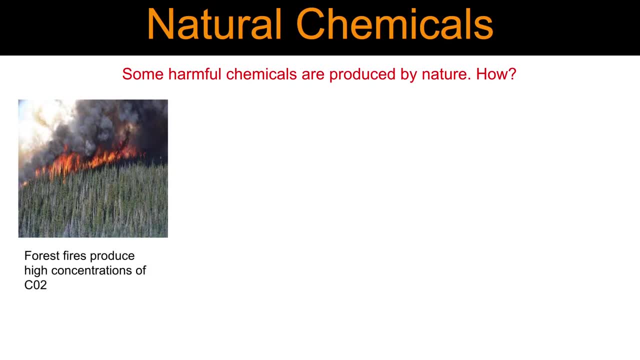 a lot of gases, so forest fires produce high concentrations of co2. carbon dioxide gas is one of the leading causes for global warming. it is a massive byproduct that we need to try to mediate in our world. the next thing that we see there natural is volcanoes and volcanoes actually. 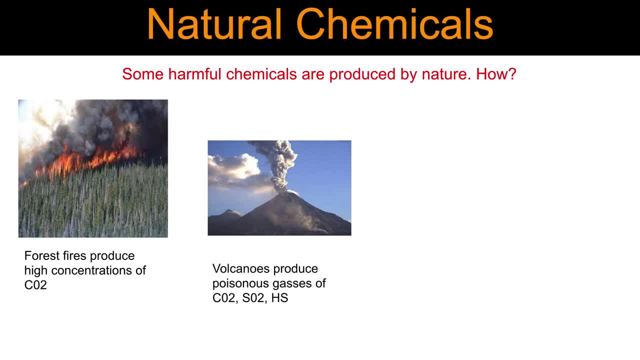 produce poisonous gases like carbon dioxide, sulfur dioxide and hydrogen sulfide- all really bad things. in fact, when volcanoes blow up, it affects the entire atmosphere, not just the place that it blows up, but even in our own atmosphere. here it will begin to pollute the world with different types of gases. we have to be really careful with that, and we 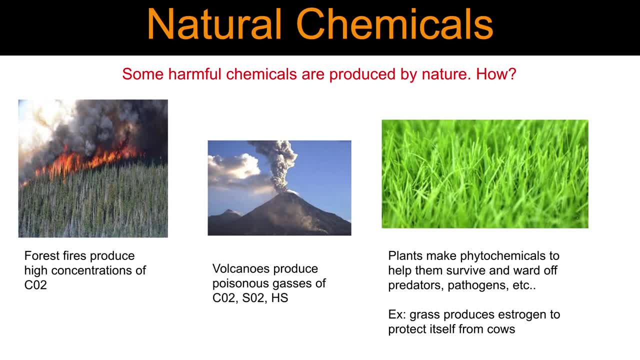 have to watch that plants make photochemicals to help them survive and ward off predators. what's interesting is, some plants are able to actually produce things inside of them to be able to keep them safe. so we have to understand that producing chemicals is something that the 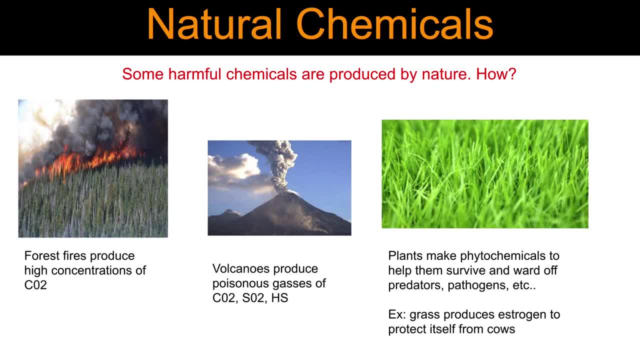 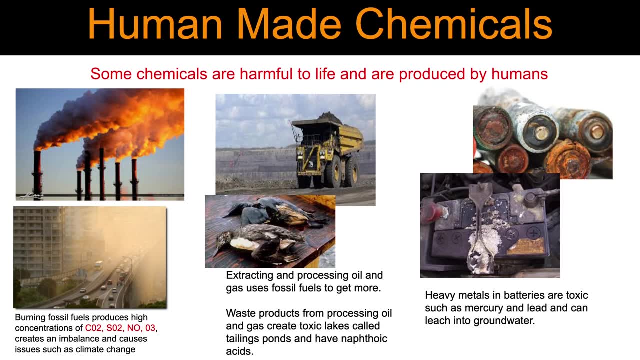 natural elements do all the time. it's what we as humans do with that and how we understand that that helps us move forward in the chemical world. some chemicals are harmful to life that are produced by humans. well, obviously you know this, so obviously you see some of the industry there. 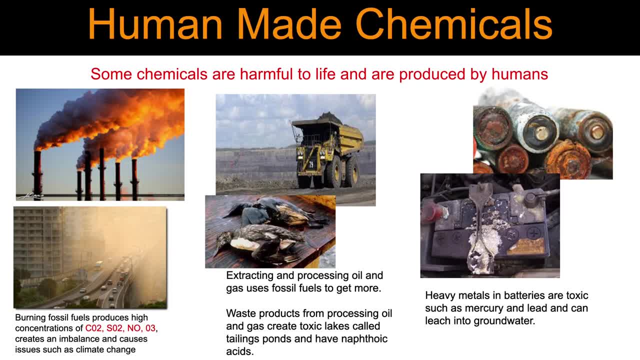 burning fossil fuels- massive thing we're going to be talking about. you have to understand that co2 is an extremely dangerous gas that goes into the atmosphere and it affects our temperature on earth. it affects how we live: sulfur dioxide, nitrogen monoxide and uh and uh o3, which is uh. ozone is super bad and it creates an imbalance which actually uh. 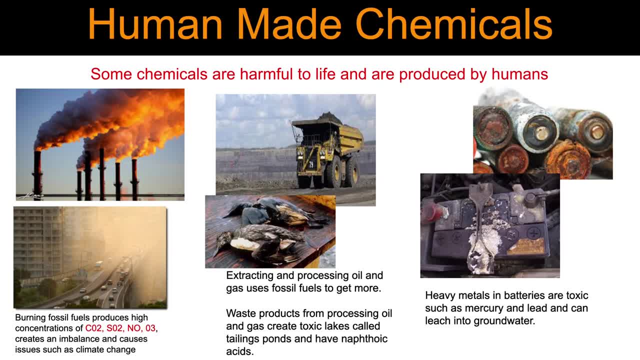 creates kind of this climate change that happens, and that's the stuff that that a lot of people have been talking about in the news, prior to all the stuff that's going down right now. um, we have some other processes there. um, extracting and producing oil and gases uses fossil. 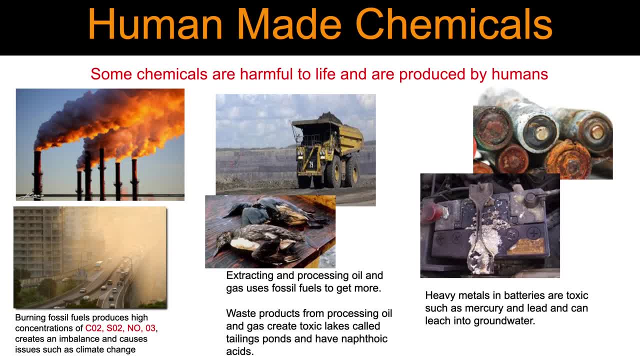 fuels to get more so. alberta uses a lot of fossil fuels. this is a really big deal here is that we could be producing a lot of byproducts that could be dangerous to the environment. waste products from processing oil and gas create toxic lakes um tailing ponds and have uh. 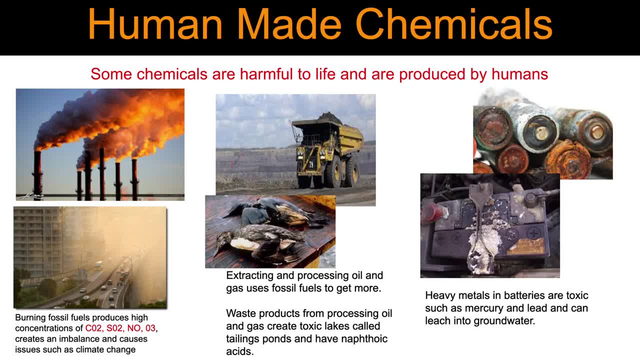 nathopathic acids, so just super bad acids, whenever we're kind of doing that. we'll look at that a little bit later. another thing that we have to be really mindful about is this thing called heavy metals, and this isn't something that we are going to look at right right now, but when we 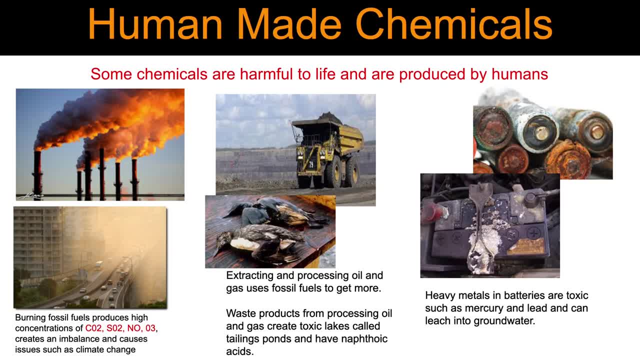 talk about heavy metals. you can see there in the picture that there's battery acid. heavy metals in batteries are toxic, such as mercury and lead. you guys, there is massive. uh, there's a massive deal that happened in japan with massive amounts of mercury poisoning. in fact, it created mutations. 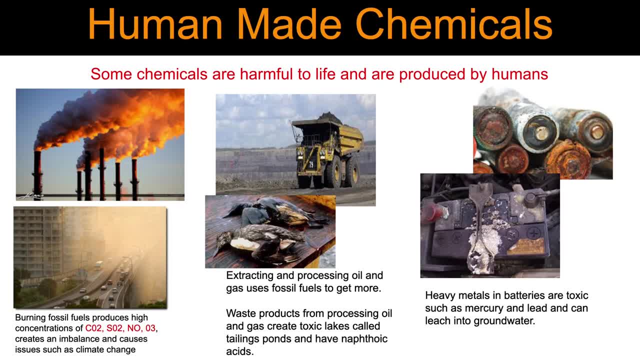 in babies, and we'll start to look at that later. but the deal is is that heavy metals, things that are actually on the periodic table, that are metals- can be super dangerous to humans if we ingest them in any way, shape or form, and those metals can actually get into the environment, into the rivers. 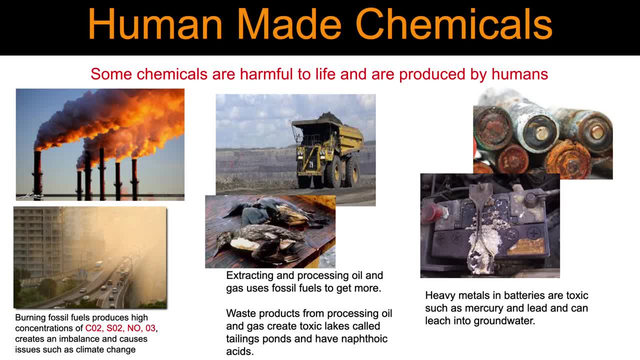 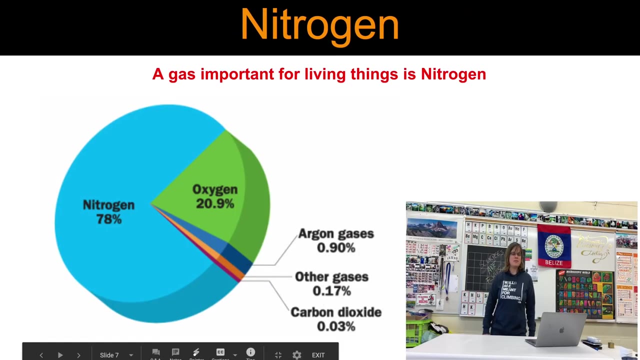 into oceans and we need to be able to be careful with that stuff. so those are dangerous things that uh, that we can make them or reuse them in our products, throw them into a landfill and then they leach into the atmosphere and that's not good. so the next thing that is uh is important. 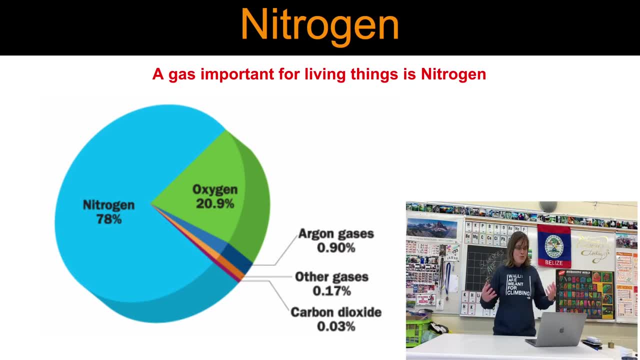 for us to understand is nitrogen, and nitrogen is a huge piece of the air that we breathe. if you're taking a look at the chart right now, you can see that nitrogen makes up 78 of the air. this is something that you're going to have to understand. 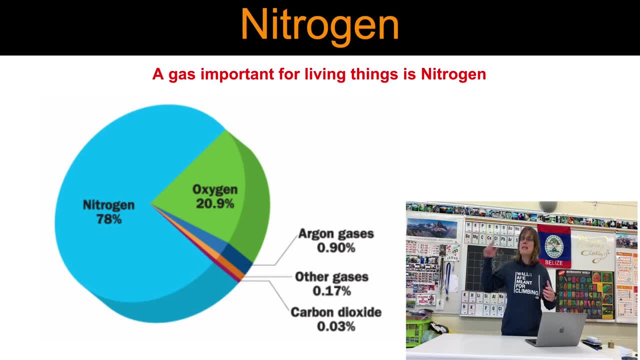 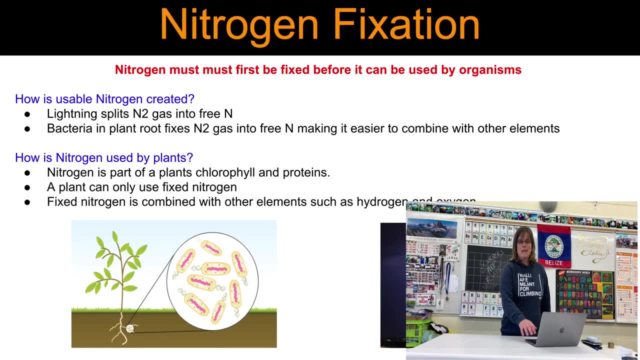 next year and the year after. the deal is is that nitrogen is in the oxygen that we breathe. but nitrogen is actually unusable in its form right just like naturally in the air. so nitrogen has to be fixed. we call it not fixed like you fix your puppy or anything like that, but it actually just 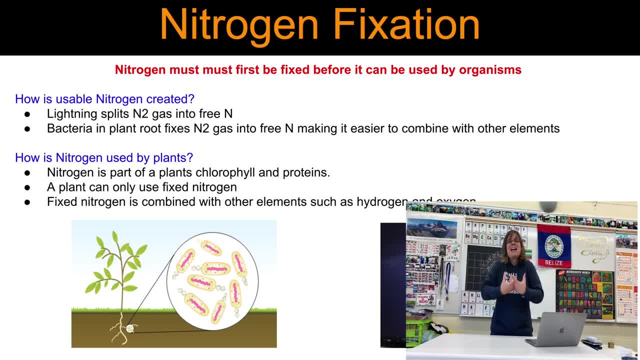 has to be uh created to to be able to attach to things, to be usable. nitrogen in its form, just n2, it comes like that in the atmosphere. what um? it needs to be fixed to be able to do things inside of plants. it needs to be fixed to be able to be usable in our world. so how is usable nitrogen? 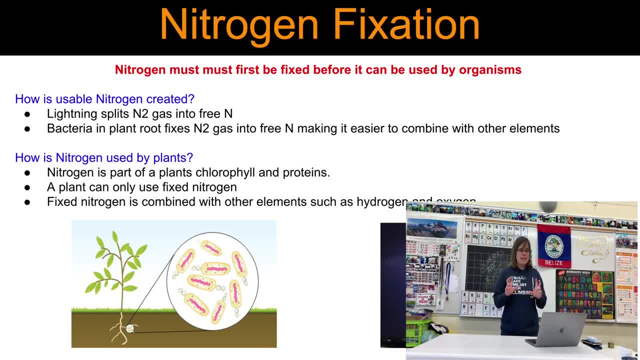 created. so what's really interesting is that a natural process like lightning- this is super crazy- is that it actually splits the end to the nitrogen and it creates free um. nitrogen ions just ends. see, nitrogen in the atmosphere comes in n2, but actually, uh, we want to free it into just being an. 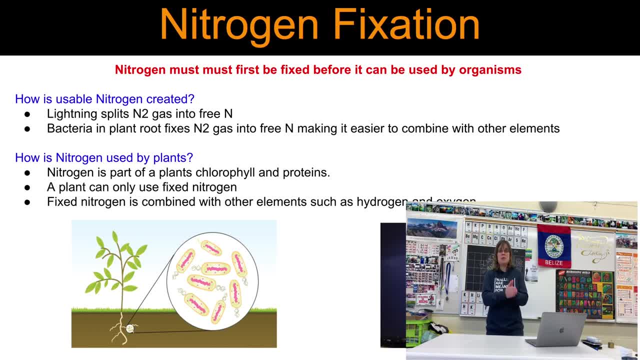 end. bacteria in the atmosphere comes in the atmosphere and nitrogen comes in the atmosphere. in plant root actually fixes nitrogen to be usable by plants. um, and so there's this bacteria in the roots that actually fixes the nitrogen in the air and allows plants to use that nitrogen to grow. 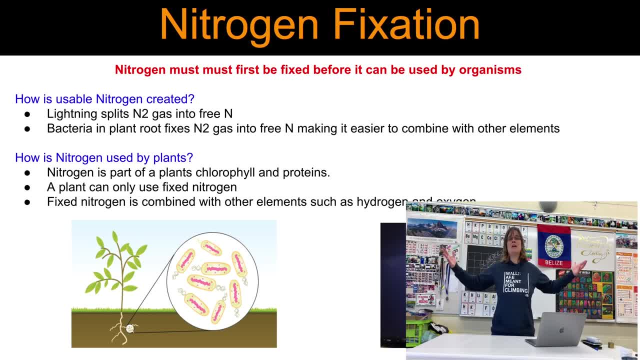 nitrogen fixation is important because nitrogen in the air is unusable until things like lightning and things like plant roots actually combine together to make those elements useful in our bodies or useful in the plants or useful in the atmosphere. so why is nitrogen important? this is something that you're going to look at in grade. 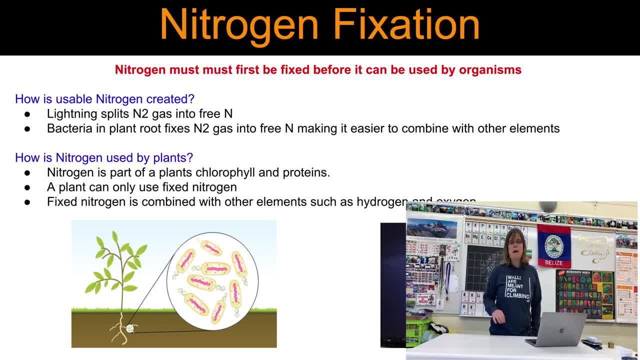 11 science relatively briefly, but also comes back to you if you do biology in grade 11.. um, nitrogen is part of a plant's chlorophyll and protein, so nitrogen is important in plants. in fact you find in fertilizers, which we'll look in a second. a plant can only use nitrogen. that's been fixed. 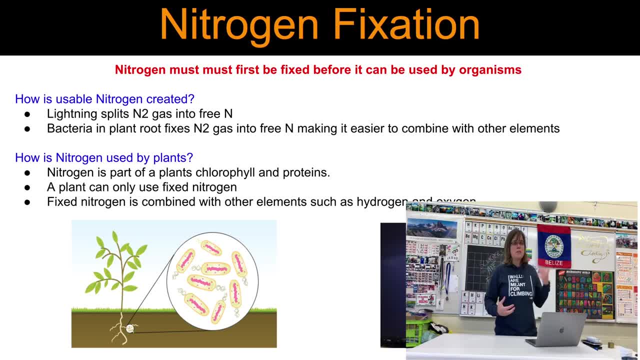 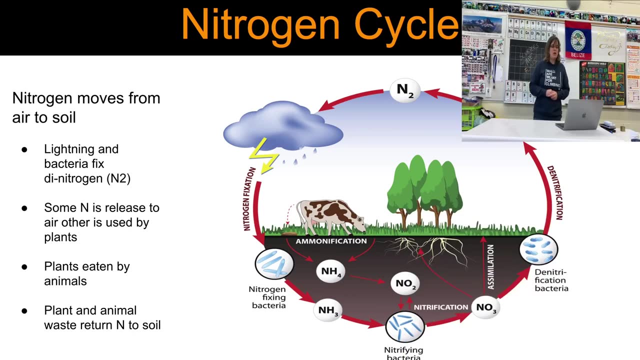 so nitrogen that's been, uh, you know, either fixed by the roots or fixed by that lightning, because if you can't don't fix that nitrogen, you just can't use it. so fixed nitrogen combined with other elements such as hydrogen and oxygen get fixed and then actually it creates this cycle. the nitrogen cycle has to do with how. 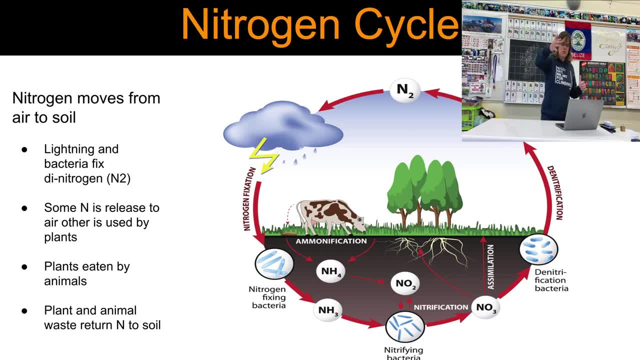 the nitrogen moves from the air down into the soil, all the way down to the depths of the soil, and then how it comes back out of the soil and gets used again in the atmosphere and it keeps cycling. an important cycle for you to understand if you take a look at there. um, the when, the 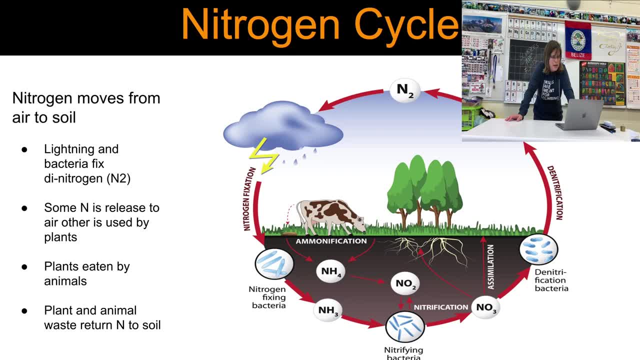 nitrogen is in the air. it's actually fixed by the lightning bolt there, which means that it's being able to be used now as nitrogen when it gets into the soil. there's nitrogen fixing bacteria and that nitrogen fixing bacteria allows plants to grow because it needs nitrogen. but you 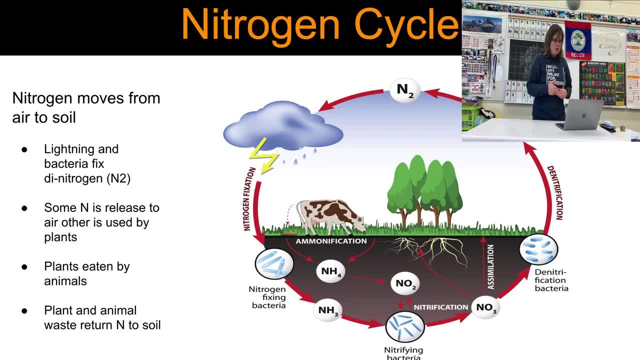 can't just use nitrogen in the air. you have to fix it. so nh3 and nitrifying bacteria actually create these different types of ammonias that allow plants to grow really, really well. nitrification happens, but then, after all, the nitrogen is used in the soil, there's a denitrification process that 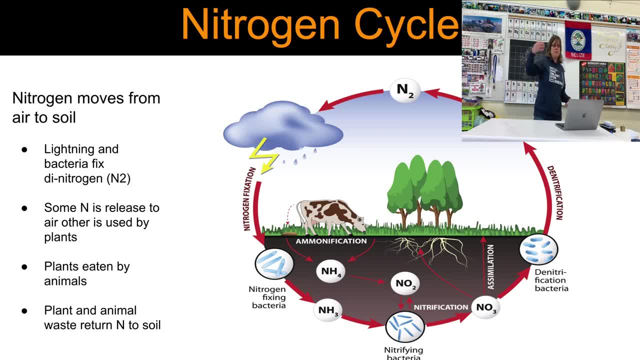 basically just means that the nitrogen goes back to being into the atmosphere and needs to be fixed again to be used again by the plants. other things that produce nitrogen for us are things like cows. cows, poo on the ground and any waste or pee that they have actually goes into the soil as fixed and 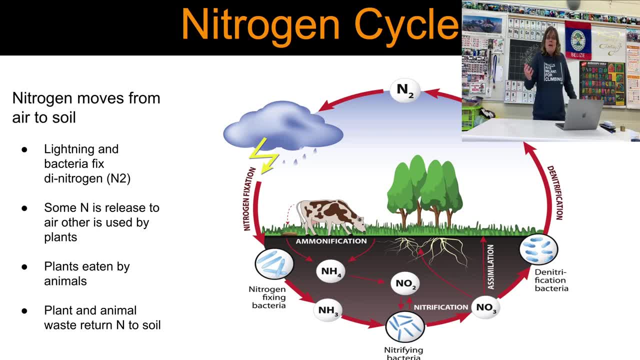 used not usable nitrogen and helps plants grow. this is why we spray manure all over the place and make plants grow, and so basically you need to understand that that when the plants are eaten by animals, they're able to fix that nitrogen and poop it out and actually it makes plants grow a lot better. 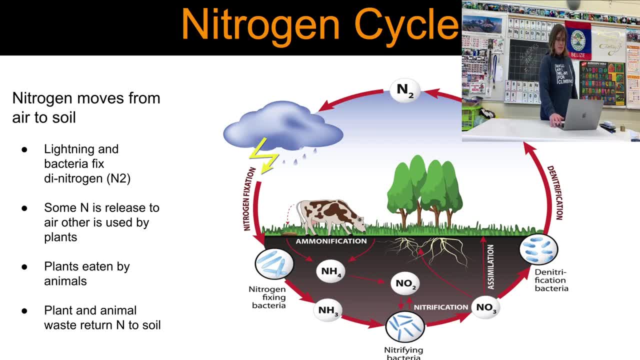 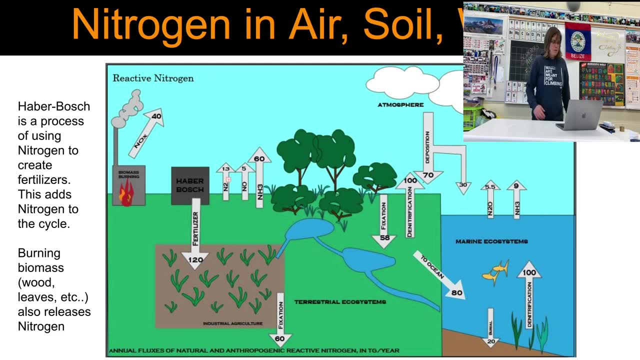 too, which is kind of crazy. so nitrogen is in the air and the soil and in the water. so there's this thing called the haber bosch, and it's a process of using nitrogen to create fertilizers. so nitrogen is in fertilizers- you need to know that- and this adds nitrogen to the nitrogen cycle burning. 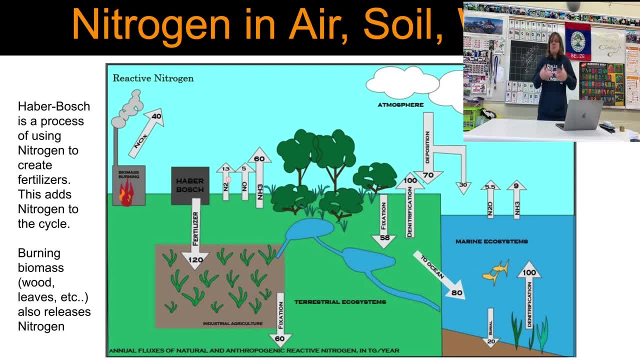 biomass, which is like burning wood or leaves, also releases nitrogen into the atmosphere. so if we take a look at this diagram, we can see that nitrogen needs to be fixed for plants to grow, as you see there. so that's why we put that nice little fertilizer in the soil that helps the plants grow. 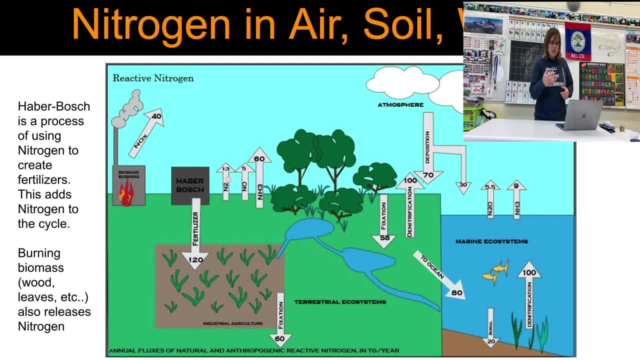 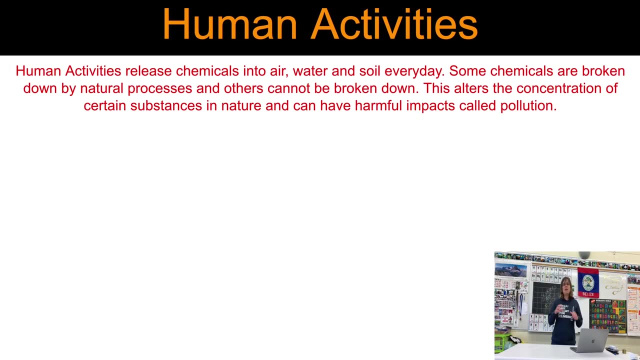 and then there's all of these things happening. some of the nitrogen goes into the ocean and then, basically, the nitrogen goes back into the atmosphere. nitrogen is cycling all over the earth into the water cycle, into the soil, all the time, and so it's just important for you to understand that it's all there. here's the deal. humans are full of nitrogen. 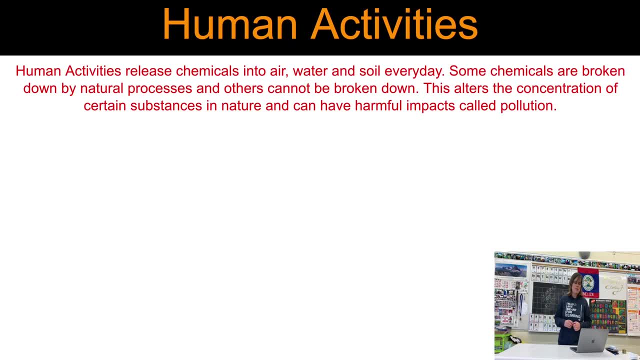 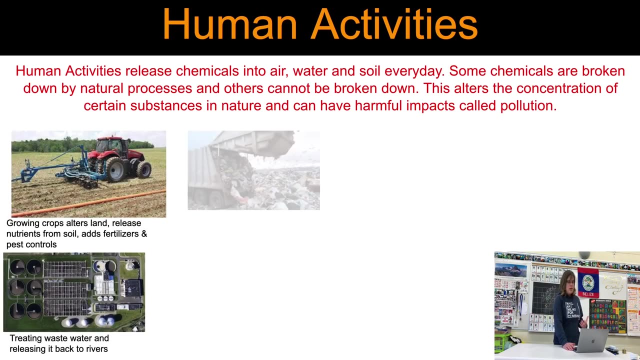 that's the environmental effect. humans release chemicals into the air, into the water and soil every day. some chemicals are broken down by natural processes and others can't be broken down at all. this alters the concentration of certain substances in nature and can have a harmful impact called pollution. so, you guys, here is all of the pieces that pollution adds, and this is basically. 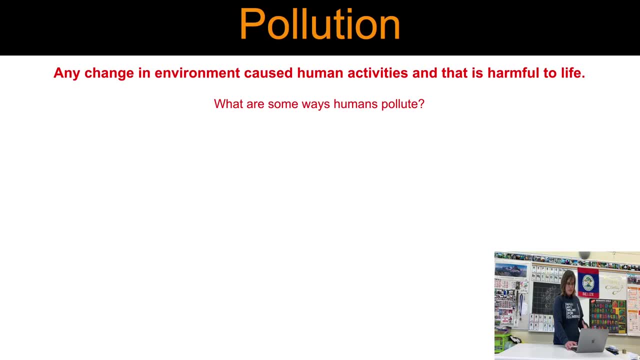 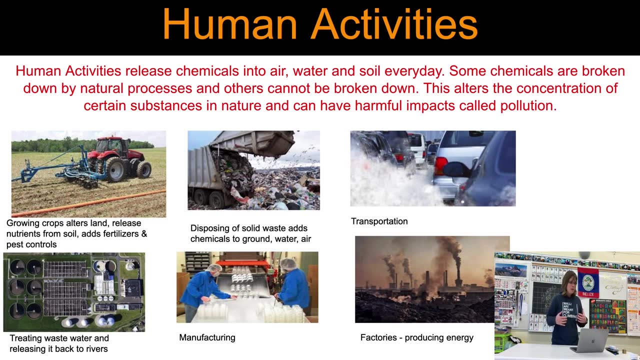 what this unit is all about is how are these dangerous gases that we've, that we've read about, affecting our world? so, basically, here's the deal with the environment. here's the deal with the. we look at growing crops and altering land releases nutrients from the soil. it adds fertilizers. 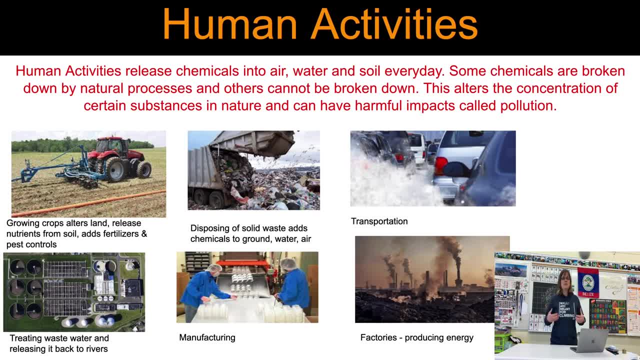 and pest controls. you guys, when we farm land, we need to use pesticides, which are chemicals that we made, which can affect the environment. when we farm land, when we put chemicals on that soil, it actually can leach into the water, and i'll show you what happened. we'll create. 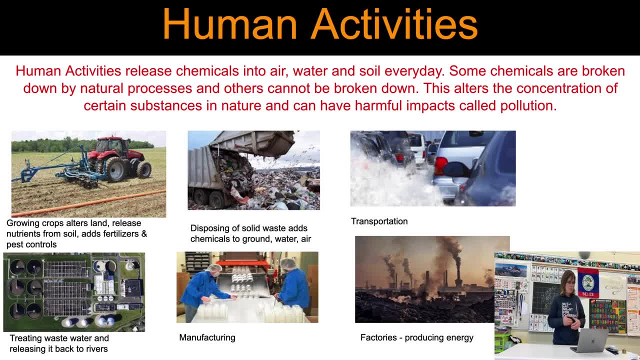 lj blooms, so that's super. not great all the time. so we have to be able to to mediate that. we have a wastewater treatment plant and treating wastewater and releasing it back into the rivers, so we have to be able to take out the harmful things and be able to put it back in. but that 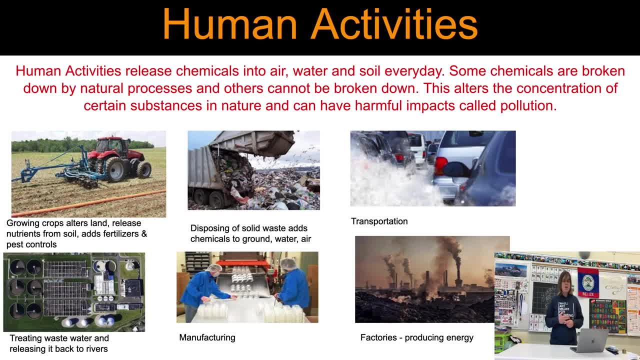 involves chemical use as well. we need to be able to dispose of solid waste. so, even like our diapers and stuff that we use to change our, our babies and stuff go into the landfills, and so we have to be able to be careful that all of that baby juice from the diaper doesn't. 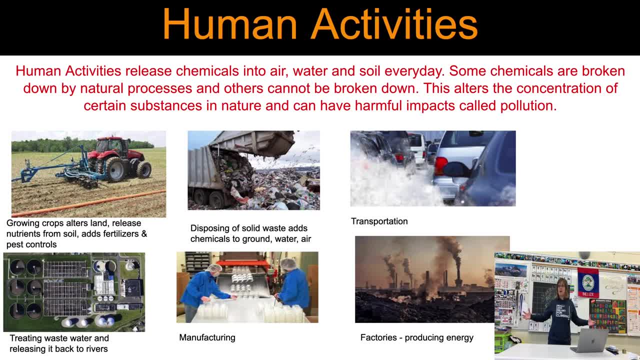 seep into the soil and affect what's going on in the environment around them. manufacturing produces tons of gas. you've seen it all the time. you've seen those big stacks and stuff like that- and it releases gas into the atmosphere. and that is manufacturing. we have to make goods, but when we make goods we make gases. transportation is a huge one, which is 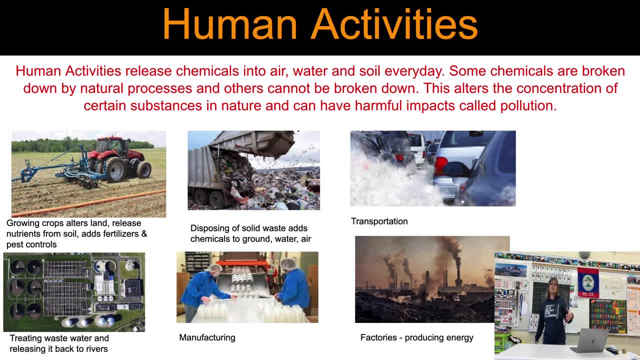 why they don't want us to drive our cars around or why they're making hybrid cars so it doesn't take as much gas and it takes some electricity. we don't want to release harmful chemicals into into the atmosphere and factories, like we said in manufacturing, produce tons of gas into the. 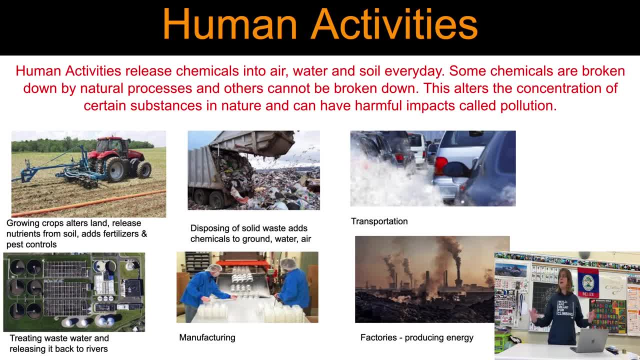 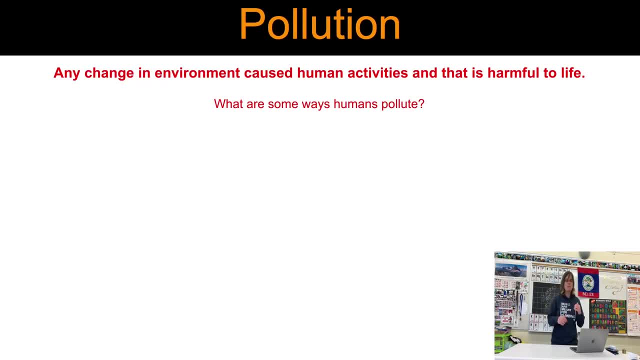 atmosphere, which again affects global warming, which again can affect really just how our atmosphere is reduced responding. so you need to understand that pollution, any change in the environment caused by a human activity, is harmful to life. so what are some ways that we pollute stuff? well, if we take a 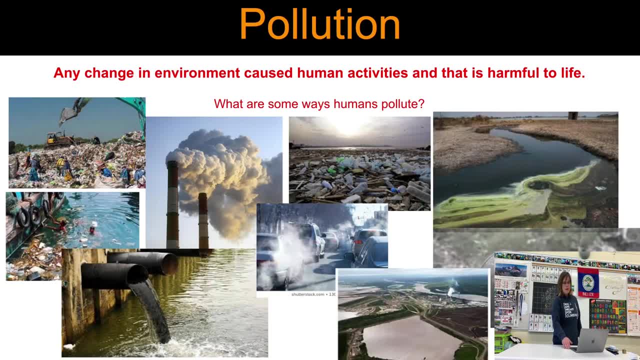 look at all these pictures, we can see that there's tons of ways that we are polluting the environment every day. obviously we look at like things like plastic bags, or we look at things like stuff that doesn't biodegrade. we're trying to to move away from those things and and lessen our 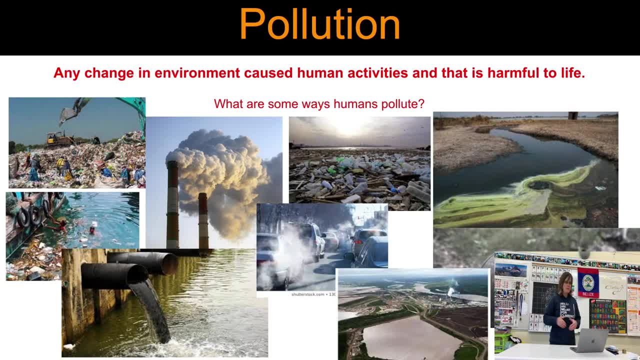 carbon footprint. we're looking at gases that are releasing into the atmosphere from factories. we're looking at water that goes back into the lake. if you go for a bike ride or for a walk by the river valley, you'll notice that there's all these like crazy things that release water back into the. 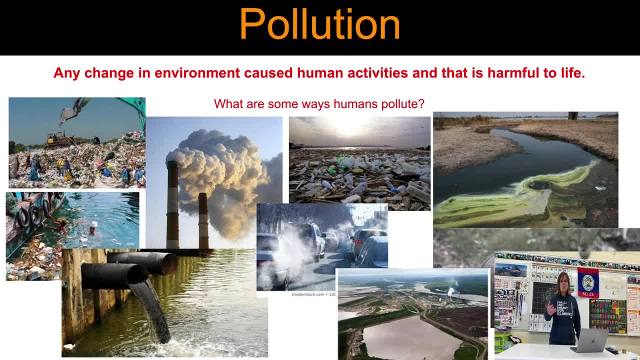 into the atmosphere, to the to the north saskatchewan river. is that water safe or isn't it? where is it coming from? we're driving our cars every day, we're releasing gases, um, and so on and on it goes. we pollute the environment. so we need to have focus on a few things today, so that you'll 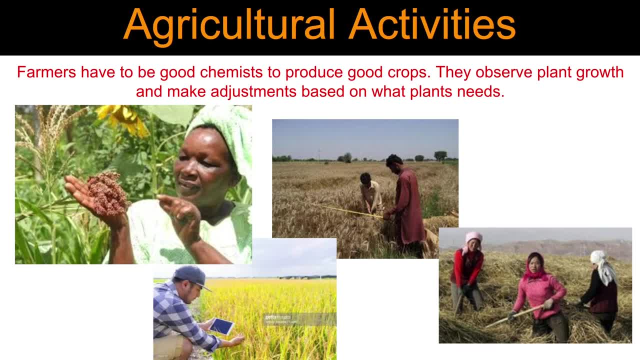 know how to do your project in this unit, and the first thing is agricultural activities. so farmers need fertilizer to produce good crops. they observe plant growth and make adjustments based on what plants need. you guys. plants need fertilizer to help them grow. we want to be able to produce the best. 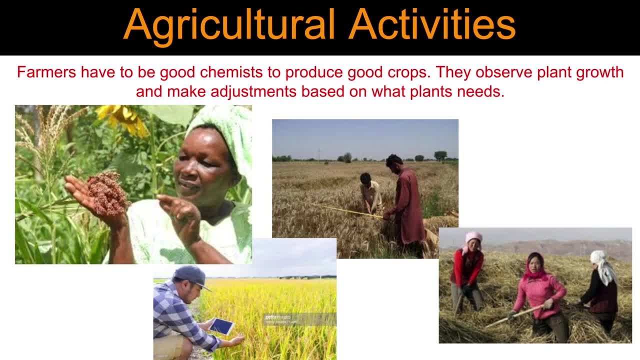 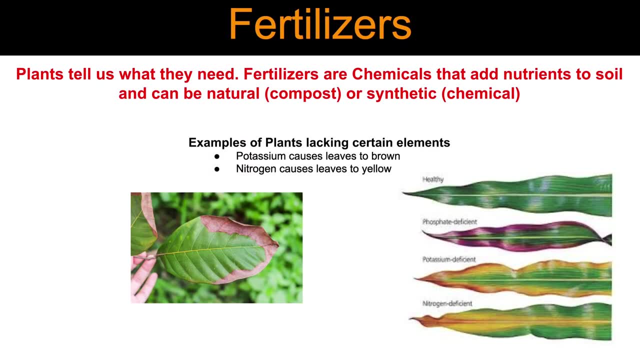 crops so that we can make, a- the most money and, b- we can feed our populations. but they're going to have to be able to figure that out and weigh that out with the environment. so fertilizers plants tell us what they need. fertilizers are chemicals that humans add into the environment. 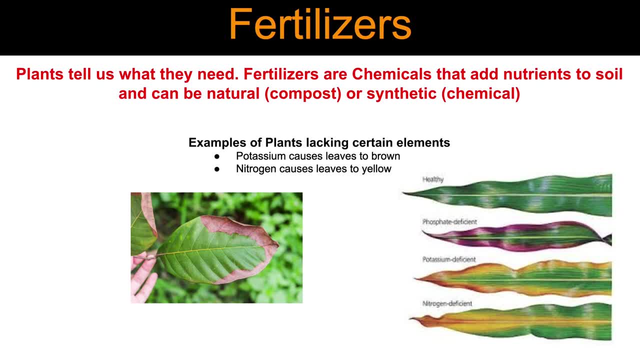 but they add nutrients into the soil and it can be compost or synthetic or something like that. so examples of plants lacking certain elements. so there you go, if you ever wanted to know what a healthy plant looks like and what other. potassium deficit, nitrogen deficit- um, actually, these three things are in fertilizers: the nitrogen, potassium and phosphate. so you can. 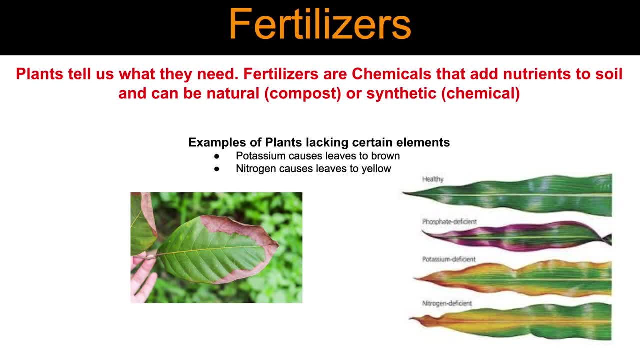 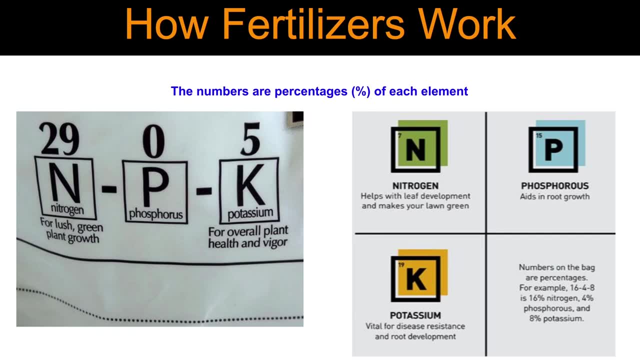 actually take a look at leaves if you are going to be like a botanist type person and figure out what they need. so this is what fertilizers do. there's always npk in fertilizers: nitrogen, phosphorus, potassium, and how much of that. when you go to the store with your parents and you're 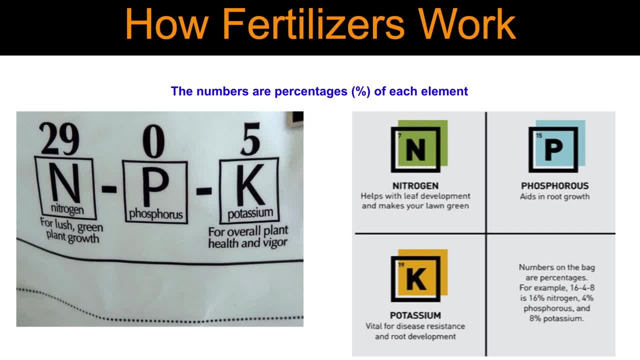 doing some gardening right now. they actually have the npk on all bags of fertilizer, and so, guys, this is what it is. nitrogen helps with leaf development. so if you have plants that you want leaves to grow, you want a high nitrogen content. it makes your lawn green, so we're going to put nitrogen into. 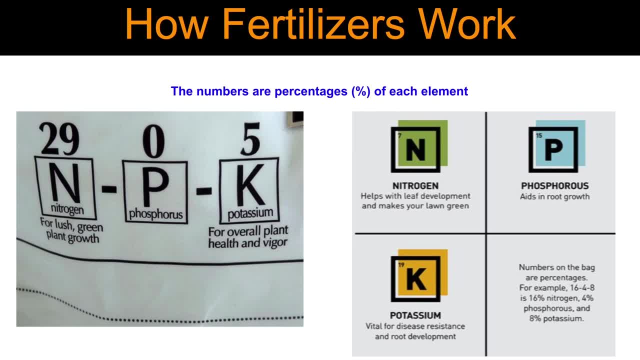 our lawn to make it green. phosphorus aids in root growth, so if you want your plants to be stable, to be able to be there for a long time, you want some root growth, and potassium is vital for disease resistance and root development. so sometimes in areas where there's a lot of 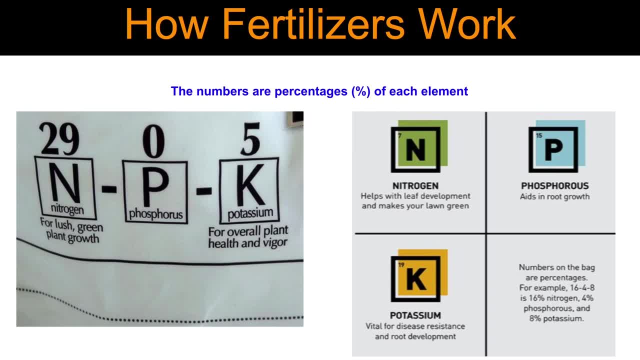 in areas where, uh, maybe the climate's a little harsher, um, and maybe there's different bugs or different things that are going on. you want more potassium. numbers on the bag are percentages. for example, sixteen four, eight is sixteen percent nitrogen, four percent phosphorus and eight. 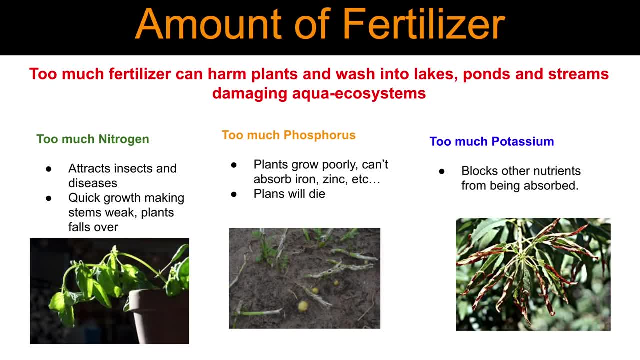 percent potassium. so, guys, this is a big one. too much fertilizer: what does it do? too much fertilizer can actually harm plants and wash into lakes, ponds and streams, damaging um aqua ecosystems. so if you nitrogen um in your fertilizer, it attracts insects, which we don't like, and lots of diseases it makes. 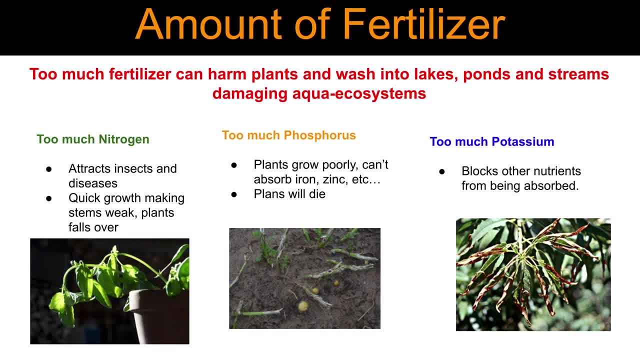 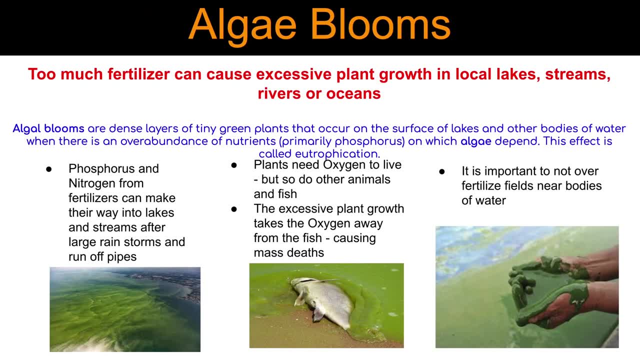 things grow um quick, making stems weak and plants end up falling over. if you get too much potassium, the plants grow too poorly, they can't absorb zinc, and if you get too much potassium it blocks other nutrients from being absorbed. something that we talked about lots in class when we were here is 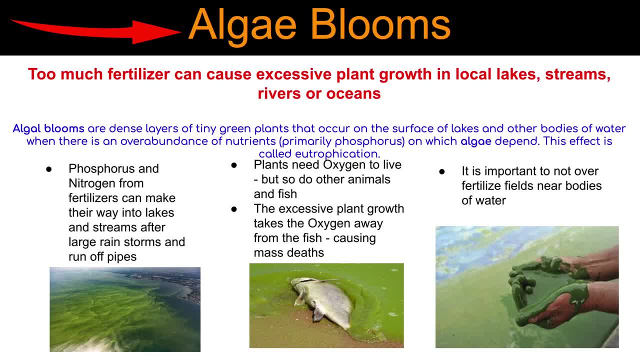 is lj blooms. too much fertilizer can actually cause excessive plant growth in local lake streams and rivers and oceans. lj blooms are something that is uh most human cause because of fertilizer. lj blooms are dense layers of tiny, thick green plants that occur on the surface of lakes and other bodies of water where there's an over abundance of nutrients. 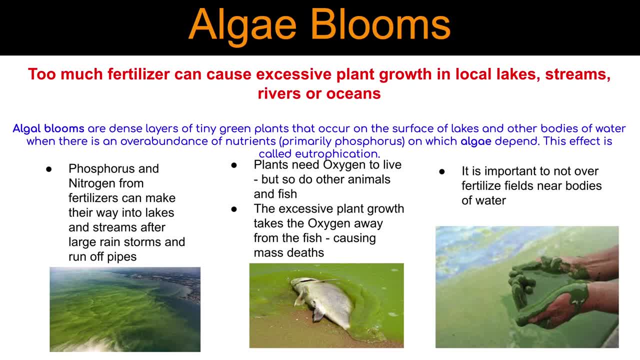 primarily phosphorus from fertilizer, on which lj depends. this effect is called eutrophication. you guys, this happens in our alberta lakes. it's part of the reasons why our alberta lakes are sort of gross and disgusting to go swimming in. so phosphorus and nitrogen from fertilizers can. 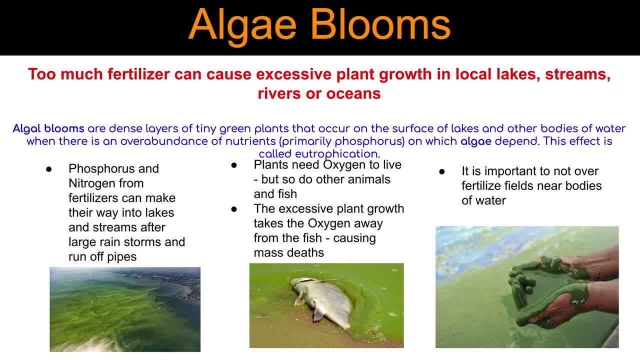 make their way into lakes and streams after a large rain storm and they can run off and die. so if you look at the picture there, that is actually the ocean. and if you are going to fertilize your lawn, or if a lot of people are fertilizing their, their golf courses and all 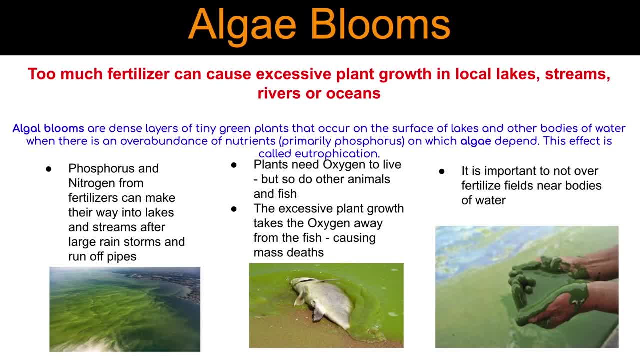 this stuff. it actually, when it rains, it dissolves all that that fertilizer and it runs off into the river and creates this massive lj bloom. taking a look at the picture next to it, it says that plants need oxygen to live, but so do other animals and fish. when you get all that green gunk inside, 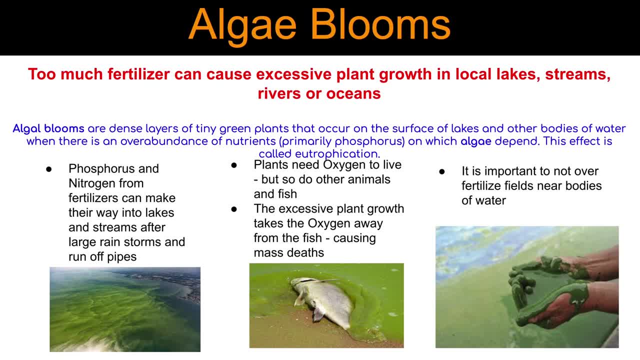 of your lakes or inside of your ponds or even inside the ocean, you're going to get a lot of oxygen. all the fish cannot breathe because the plants are taking all the oxygen. so all of the uh, all the fish die off because they have no oxygen to breathe, because all of that lj is. 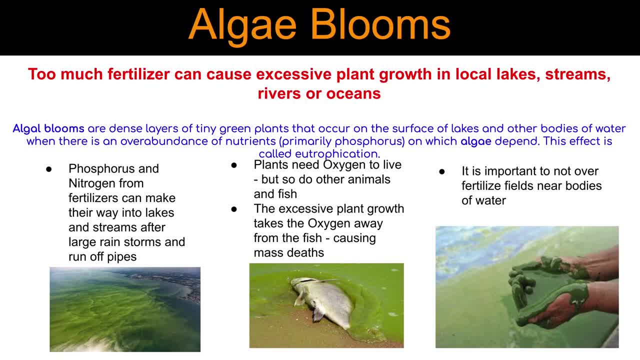 taking it away from them. it's important to not over fertilize your fields and your bodies of water, because when it rains, it can leach into that system, which is why, even in edmonton, we have to be careful, because we have a lot of golf courses along our river valley and we have 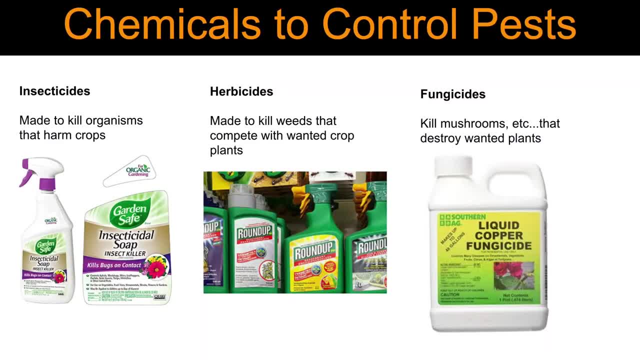 to be careful to not over fertilize so that it doesn't run into our rivers. the next thing that's important to understand about chemicals in the environment is that we use pesticides and or herbicides, so insecticides are made to kill organisms that harm crops. so lots of insecticides. 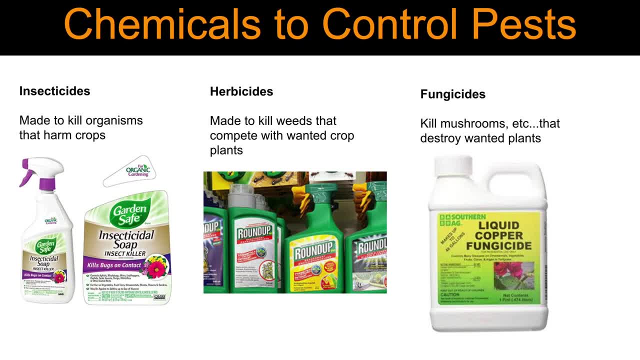 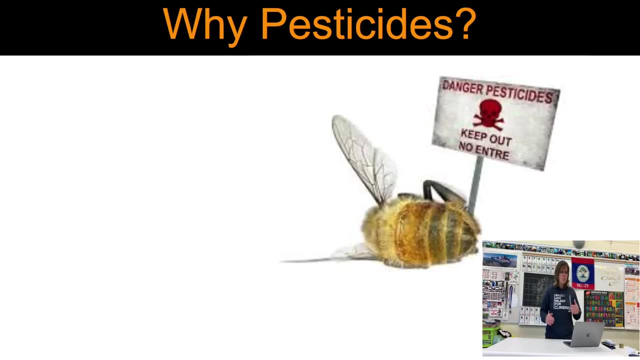 or we call those pesticides same thing: pests, insects- interchangeable word- herbicides are made to kill weeds, that can that compete with unwanted plants. so there you have a whole bunch of roundup and stuff and fungicides kill mushrooms and stuff that that destroy um wanted plants. so why do we? 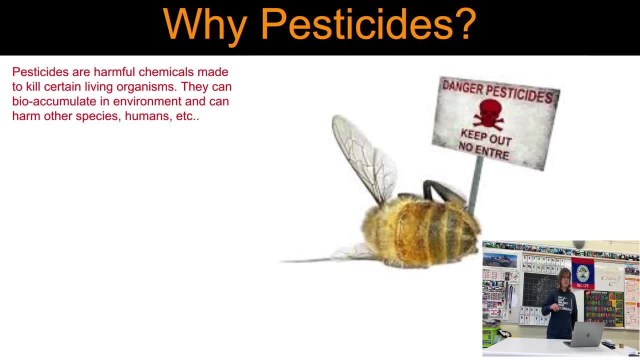 pesticides are harmful chemicals to kill certain living organisms and they can bio accumulate in the environment and harm other species and other humans. you guys, pesticides are sprayed on everything that we eat. if you're not buying everything organic, you're eating pesticides, which is why your parents tell you to wash your vegetables really, really, really well. 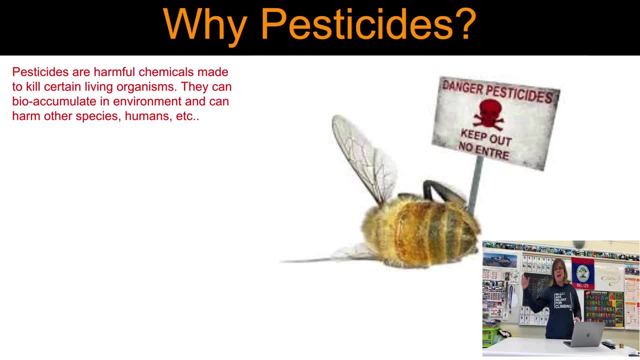 when you get them in the house, because we spray stuff so that the pests don't eat them all the time. the word bio accumulate- we'll look at that in a second- means that we we start to put chemicals on the ground on the very initial piece that we start to eat, which is our vegetables. 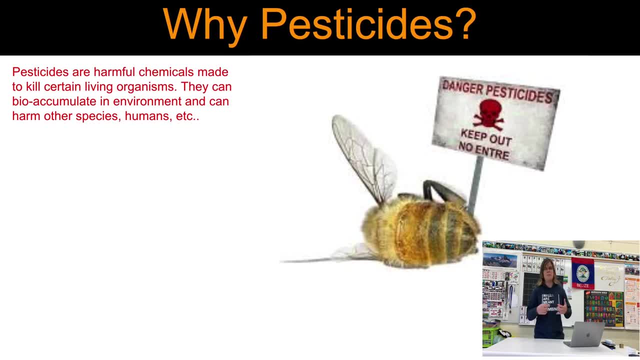 and our food and our grass. everything that we know eats that bunny rabbit. we know that. but what eats bunny rabbits is maybe a fox, and and what eats foxes is maybe a bear. and it starts to accumulate in all of the different animals up the food chain so it eventually gets to me or to you. 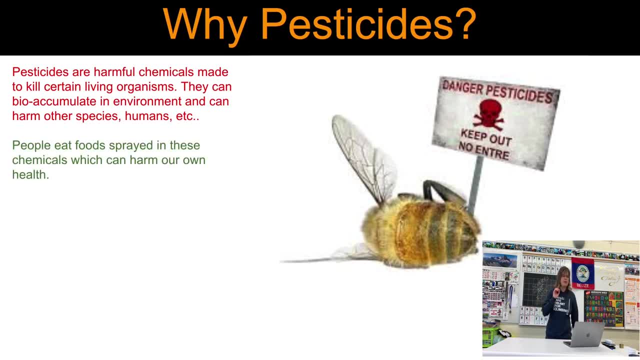 and it gets to us bioaccumulation. people eat foods sprayed in these chemicals, which can harm our own health, which is why a lot of people buy organic, or why we really want to make sure that we wash our vegetables really well so that doesn't have pesticides on it, and we don't get that. 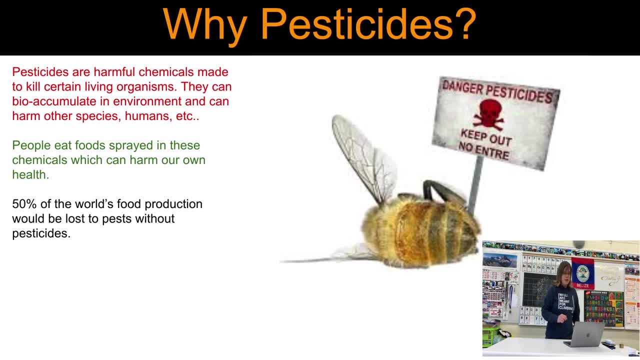 50 of the world's food production would be lost to pests without pesticides. um, i mean, guys, we have to use pesticides because think about all of the bugs that are wanting to eat our food. pesticides often kill organisms that are wanted, such as bees. so actually, what's happening? and 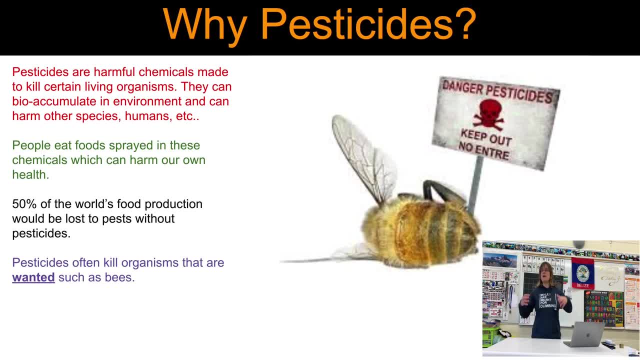 sometimes what they find is they'll put things like roundup or different stuff in their food chain and they'll put it out there and it'll die because it's going to die into their spray the wheat fields. and they'll spray the wheat fields and the bumblebees will. 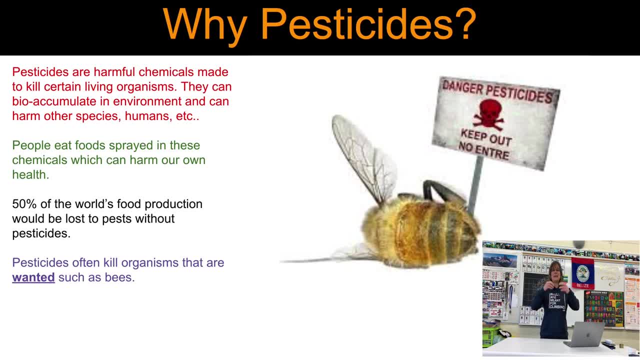 come and sometimes we accidentally create a pesticide that when the bees land and try to pollinate, they actually get that pesticide inside of them and they have found that entire bee colonies haven't made it back to their hive because they've all died because of pesticides. 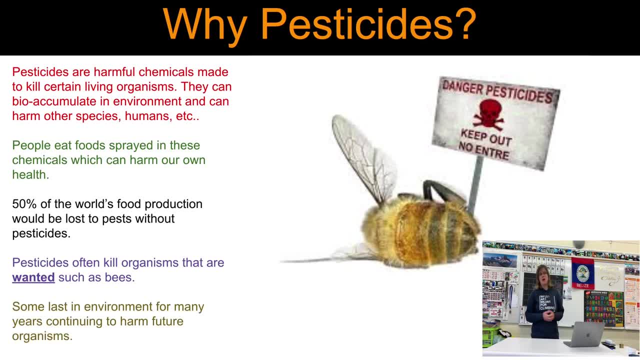 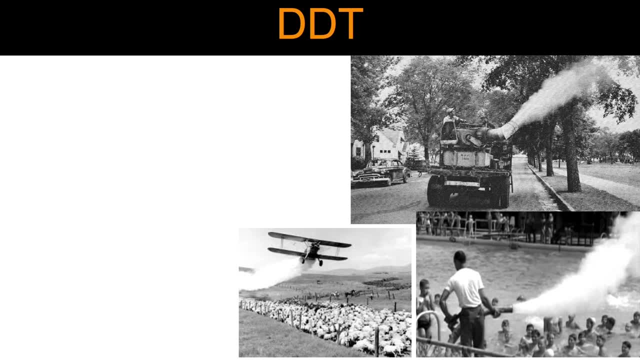 Some last in the environment for many years and they basically harm us for a long, long time, which is what we'll look at in a second. I want to look at something called DDT, and DDT is one of the most harmful chemicals that was produced that the world thought. 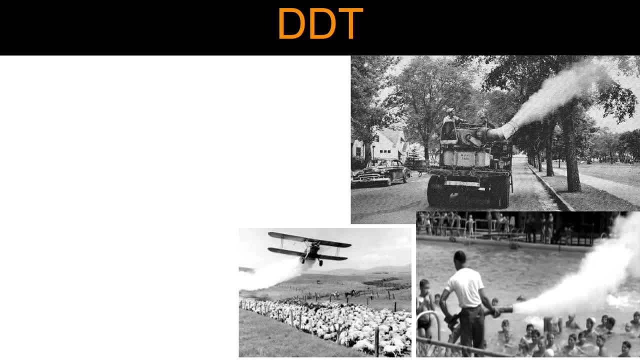 especially in North America, thought: man, this is what we need to do, This is what's going to change our lives. DDT was getting rid of mosquitoes, It was getting rid of so many different types of pests and they sprayed it everywhere, on people everywhere. It was crazy. DDT was actually created. 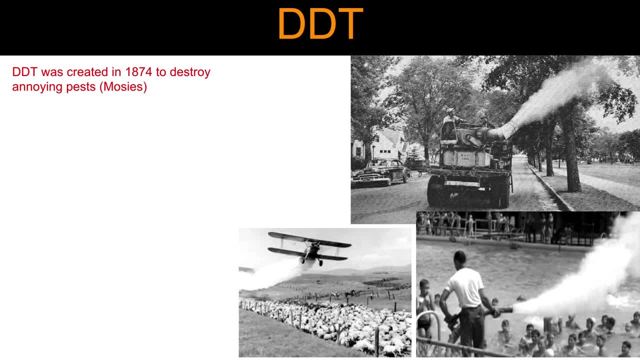 in 1874, so it's a massive pesticide that was created a long time ago and was used up into the 1900s or the early 1900s, and so it was an annoying pest and so it was trying to kill. 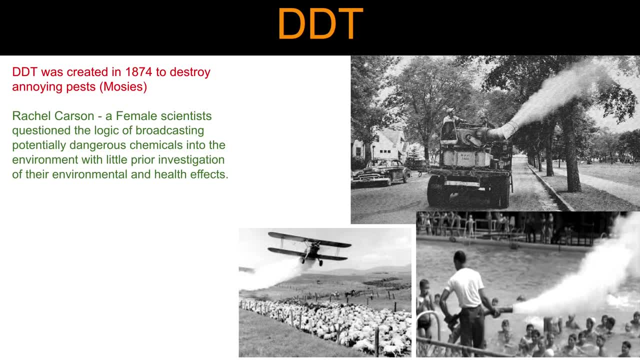 mozzies, so mosquitoes. There was actually the first time there was a female scientist named Rachel Carson. A female scientist questioned the logic of broadcasting potentially dangerous chemicals into the environment with little or prior investigation. They really didn't do very much research on this and their health effects DDT and other pesticides have been shown to cause. 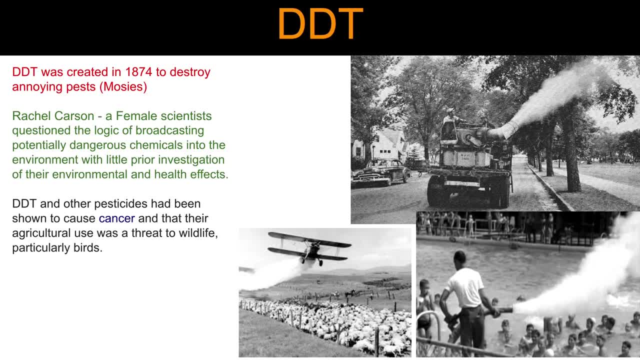 cancer, that their agriculture use was a threat to wildlife, particularly to birds. and actually what's starting to happen is, as this chemical is being used for year after year after year, more and more animals were starting to die, and in those animals we found DDT. 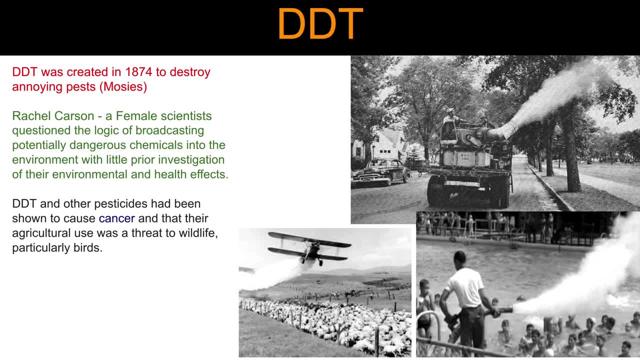 and we're talking like lots of years, hundreds of years later really, and finally this lady said: guys, we got to stop using this because eventually it's going to get into us. She was right and proved right and they eventually said: no more DDT. The reality was that, as DDT was building up, 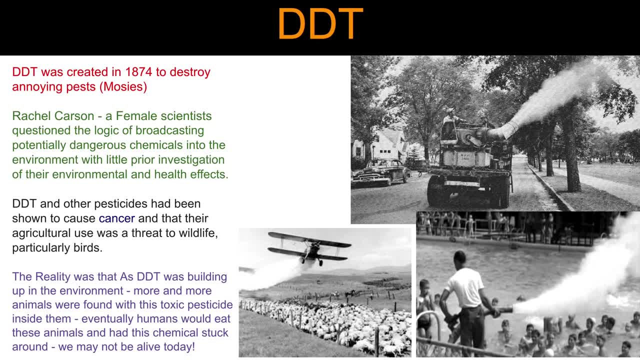 in the environment. more and more animals were found with this toxic pesticide and eventually humans would eat these animals and it would have been a disaster Today, they still do find traces of DDT in certain animals today, and that was a long time ago, If you. 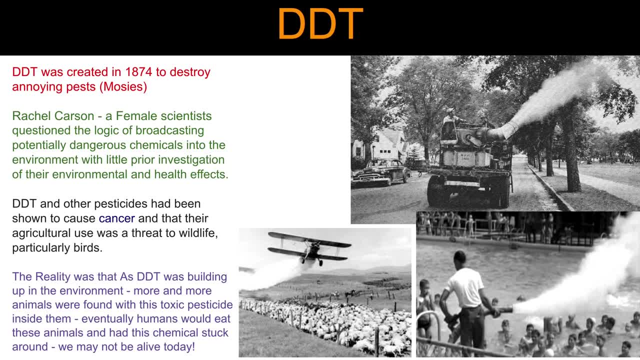 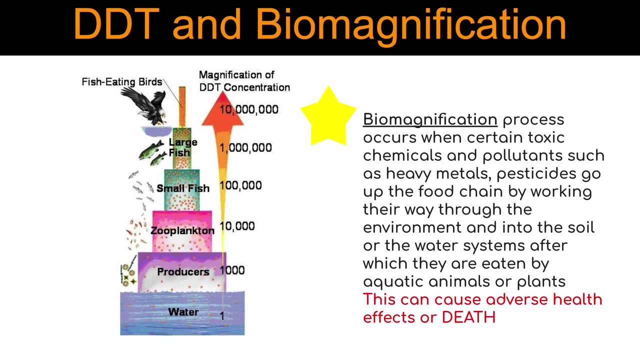 notice in the picture. one of them is a bunch of kids on a swimming pool and they're actually spraying DDT right into their faces because they believe that it would take away pests. Kind of crazy DDT and biomagnification. The word biomagnification is important to know for 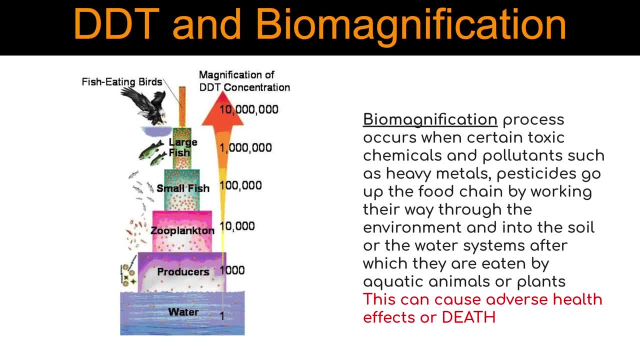 biology, and that's going to be an important word that you're going to have to understand from now all the way into grade 10 through to grade 12.. Basically, biomagnification is a process that starts to build up in the environment and it goes up the food chain by working their way through the 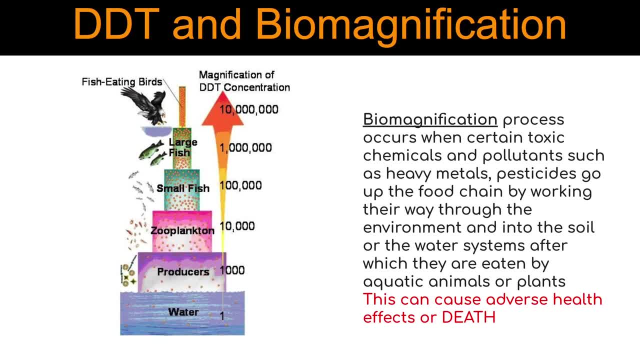 environment, into the soil or into the water system, As you see there on the diagram. you'll see that there's just a tiny bit of DDT in the water, just one part, or whatever. The producers are the things that eat the algae and they get a little bit and it starts to get more and more. 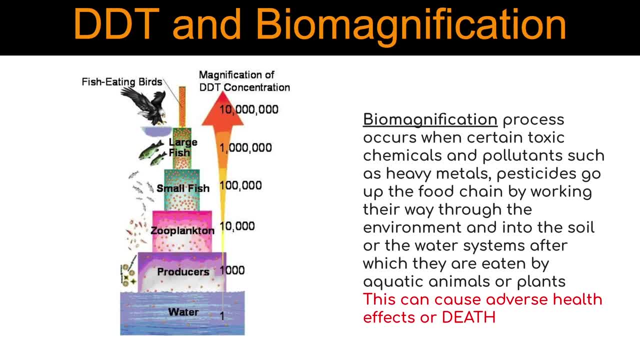 A thousand zooplankton eats the producers, so they get 10,000.. Small fish start to eat it, so it's in their body system 100,000.. We get to large fish. they start eating the small fish and the zooplankton and the producers. 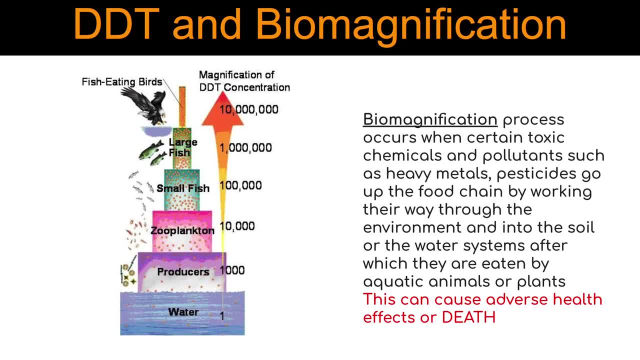 and they're in the water. so they get 1 million parts of that DDT inside of them. and then eventually that bird comes down, eats the fish and look at how much DDT is concentrated- That's biomagnification. This can eventually cause really bad health effects, or 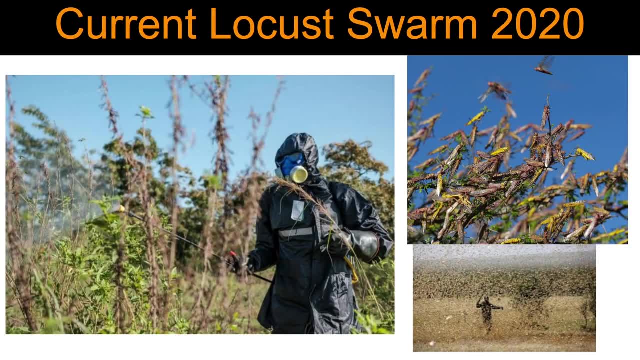 death. I want to just take a look at some pictures of the current locust swarm that's happening in Africa right now, as well as through some of the Asian countries. These locusts- it's one of the worst locusts in the world. They're very, very, very, very, very very. 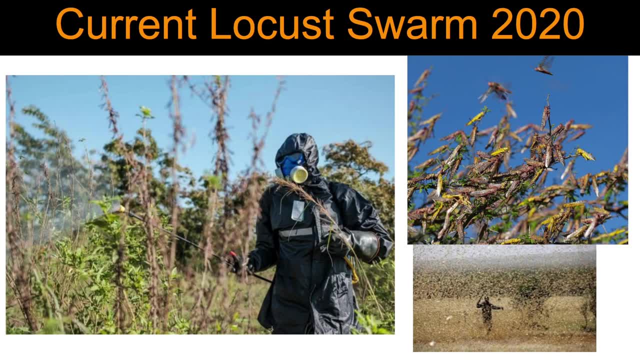 swarms, and they are millions of them. If you look at the picture in the bottom right, you'll see the man running through the field. millions and millions and millions. In fact, there's going to be more through the summer because they continue to reproduce This man. 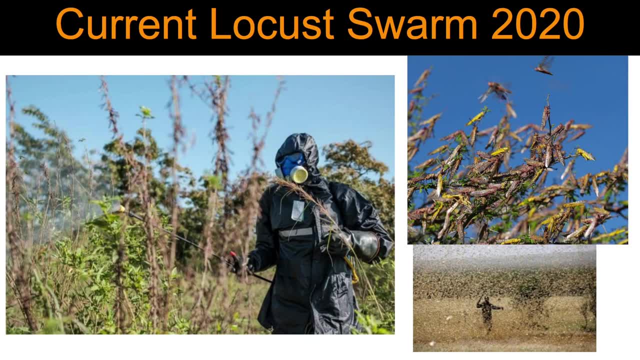 has to use pesticides to save any crop and, to be honest, it's going to eat a ton of the food down there in that different part of the world. so pretty insane. We got to use pesticides at some point, but we've got to be careful. The next type of waste that we're going to look at: 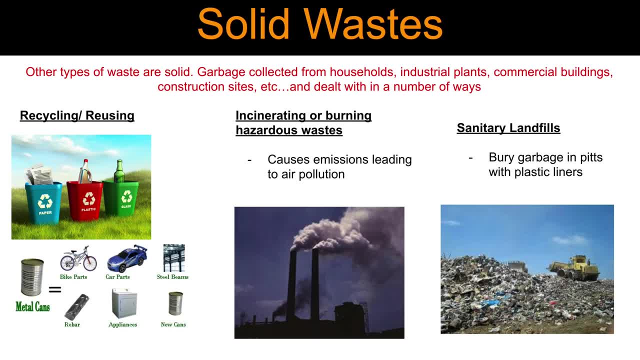 we're going to look at solid waste, so garbage collected from your household or industry plants or commercial buildings. We just want to talk just really briefly about the things you know about. Obviously we recycle stuff, Obviously in other countries, not in our country. they actually 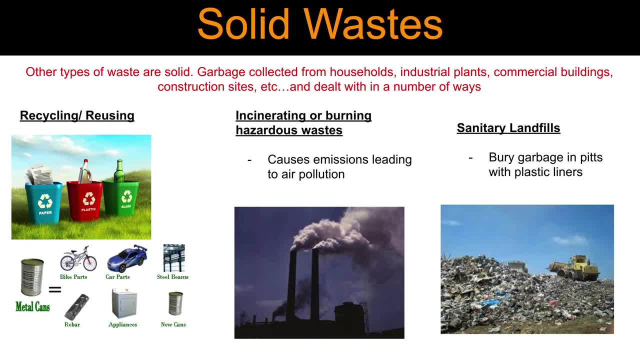 burn their garbage. Why? Because there's no space. I mean, in China, they have millions of people living everywhere, or maybe in India as well. They burn, they incarcerate their garbage. but when you burn things, you produce CO2 in the atmosphere. Basically, it can be a really, really bad cycle. 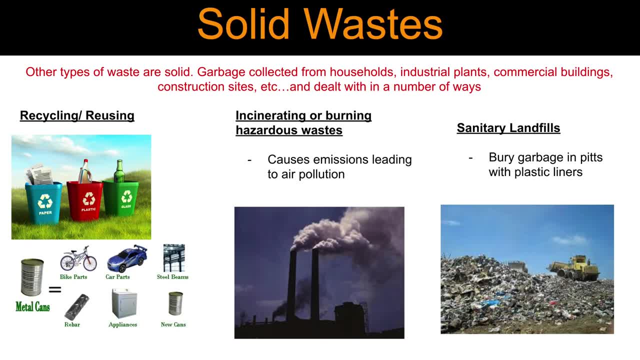 get out of hand really quickly, but it does create a lot of pollution in the air when we burn things. Sanitary landfills are what we use here in Alberta as well as in Canada, because we have a lot of space. We can dig up a hole and pour garbage in there all the time, but sanitary landfills are. 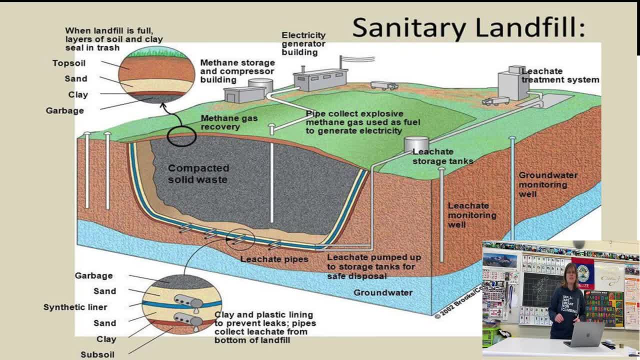 different than just normal landfills, and so let's just take a look at that. You need to understand that, when you take a look at this picture, that what you'll see is there's actually a liner, a very, really thick plastic liner that is there so that all that gross, disgusting garbage juice from 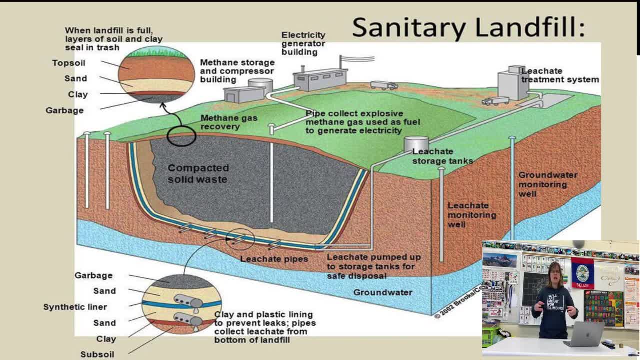 your batteries and all that stuff that's in there. it's going to be a lot of garbage and it's going to get squished out, and all of your kids' diapers as they get squished out. think about all that garbage juice that's being squished out. they want to basically protect that from getting into our 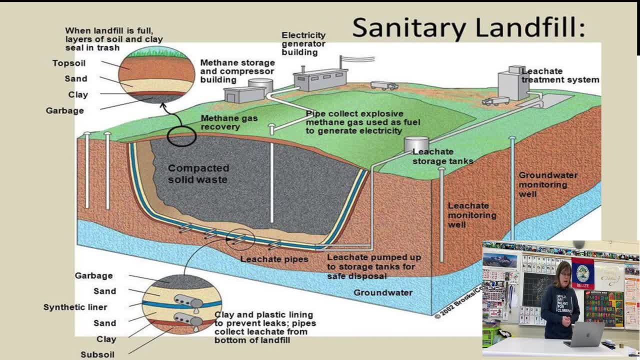 water table, which is below the groundwater that we drink, and so basically, they have these little pipelines, if you'll notice, and so these little pipelines down here called leachate pipes, and they actually pump that garbage juice into a special lake or a pool where they dispose of it. 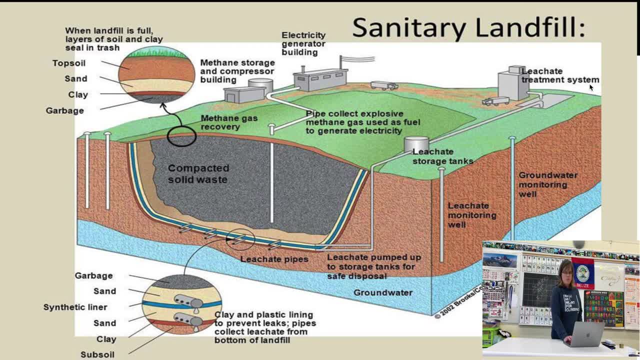 correctly, because if they just had all that garbage juice just sitting around, it would get squished out of the water and we would be drinking diaper juice, I guess. so that is a sanitary landfill having that really nice liner. You'll notice here that there's topsoil sand clay. 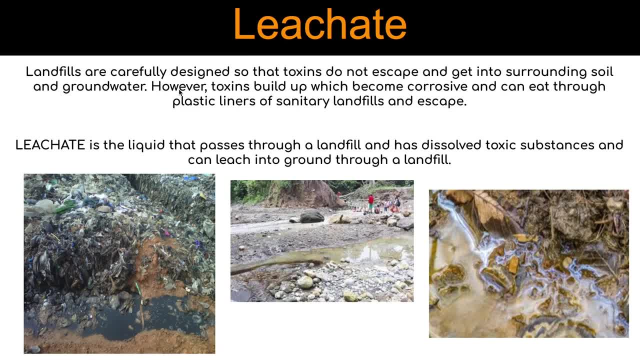 and they just have a whole bunch of different layers to be able to protect us. Leachate is garbage juice- That's just a fancy word for garbage juice- so leachate Landfills are carefully designed so that toxins don't escape and get into the surrounding soil, and so we just said that. 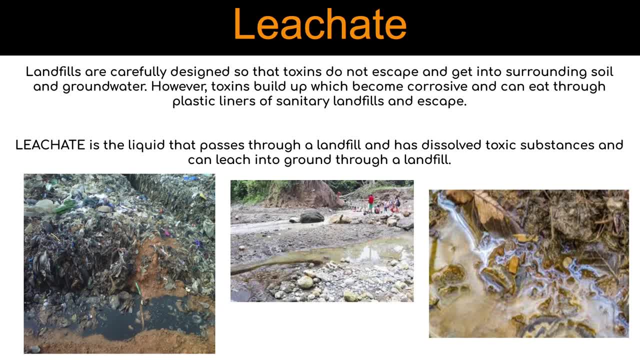 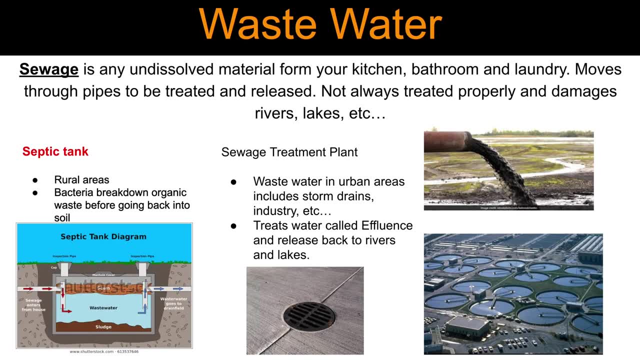 leachate is the liquid that passes through a landfill and it can leachate to the ground, and so it can be really, really dangerous. We want to get rid of it. We want to talk about wastewater like sewage treatment. so sewage is any undissolved material from your kitchen, your bathroom and your laundry. 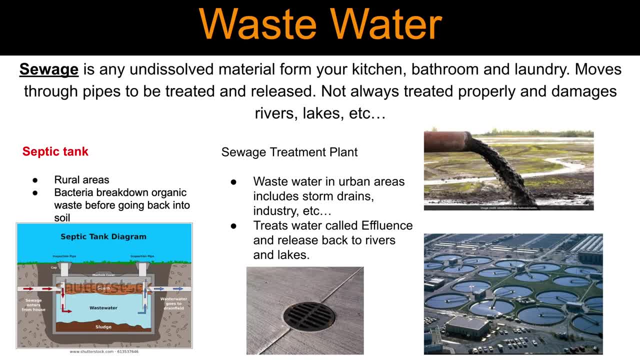 It moves through the pipes to be treated and released. It's not always treated properly and it can damage rivers and lakes. When you think about places that don't have a lot of money- and I'm talking about nations that don't have a lot of money- their wastewater treatment is a lot different. 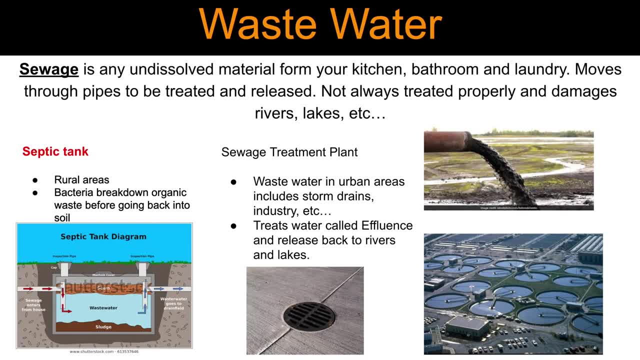 than ours is. Ours is very high, but some are very good and they just pour everything back into their bodies. They have these septic tanks that break down organic waste before going back into the soil. We have sewage treatment plants. We have a great one here. Wastewater goes into urban areas and we 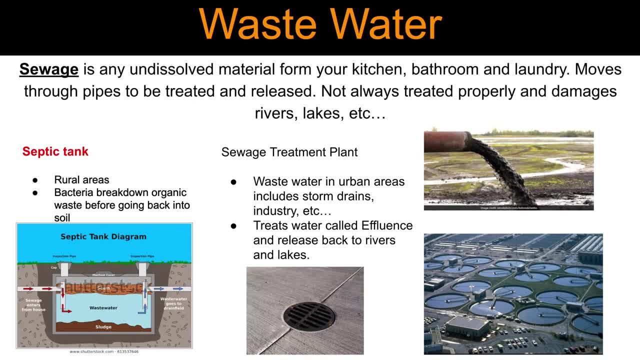 treat it and the treated water is called effluent and we put it back into the North Saskatchewan River. We drink the North Saskatchewan River, guys, so we have to be able to put the treated water, So the water that comes from your bathtub, so when you have a shower, from your kitchen sink. 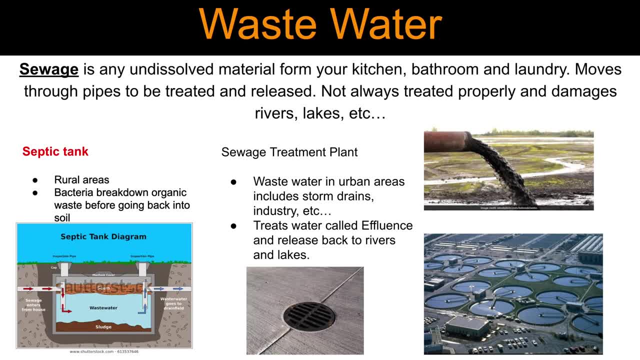 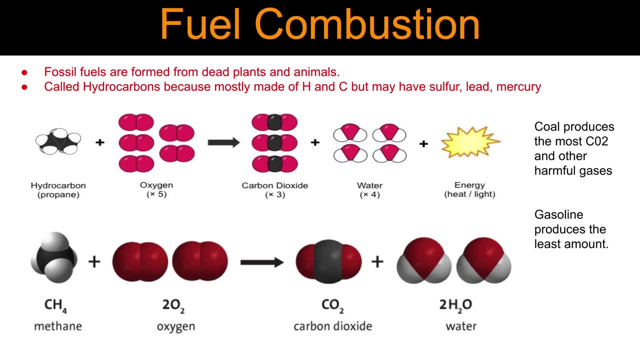 all goes to the wastewater treatment plant and then it gets pumped back out into the river as effluent after it goes through our water treatment. The last thing that we're going to talk about- that's not really great for the environment- is something called fuel combustion, which is basically happening in industries and plants. 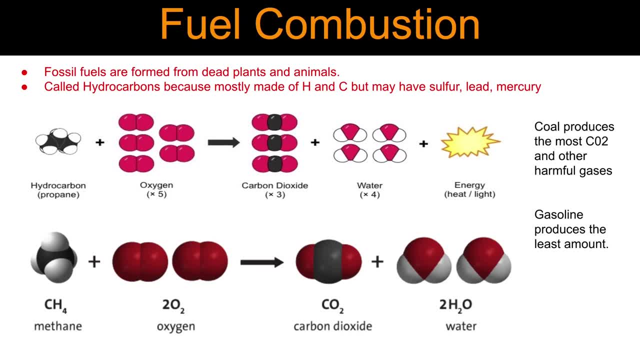 and so you'll take a look there. Fossil fuels are formed from dead plants and animals, and we have a lot of fossil fuels here in Alberta, So they're called hydrocarbons because mostly they're made of hydrogen and carbon. I call the special kind of deal as CHO, carbon, hydrogen and oxygen. 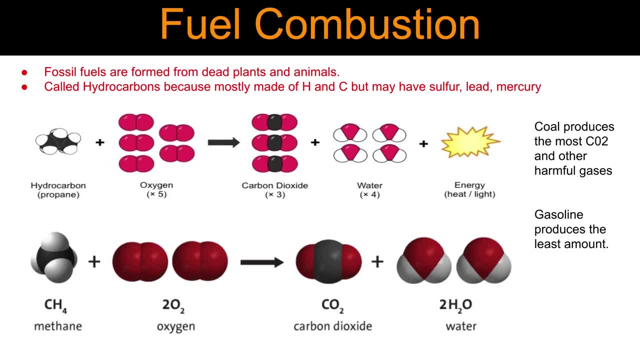 so a lot of things, a lot of gases or a lot of organic material made of CHO Anyway. so hydrocarbon here it breaks up into carbon dioxide, which we know is not good for the environment, and into water, which actually too much water vapor in the environment isn't good either It. 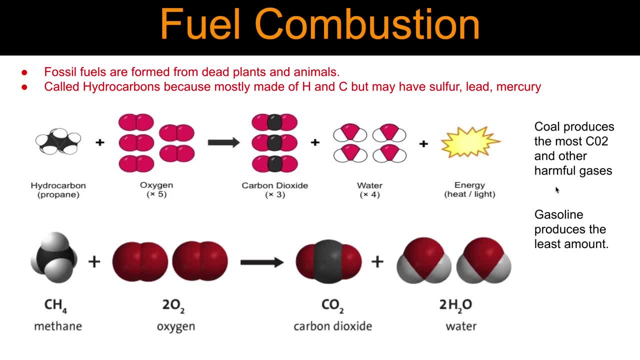 affects our climate, So coal produces the most CO2 and other harmful gases. So here in Alberta we have to be careful to process that gas and to actually make it safe to put it back into the environment. We got methane and oxygen here, and so when we have that fuel combustion there, 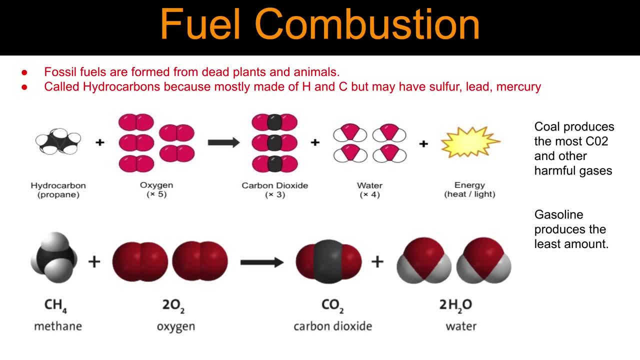 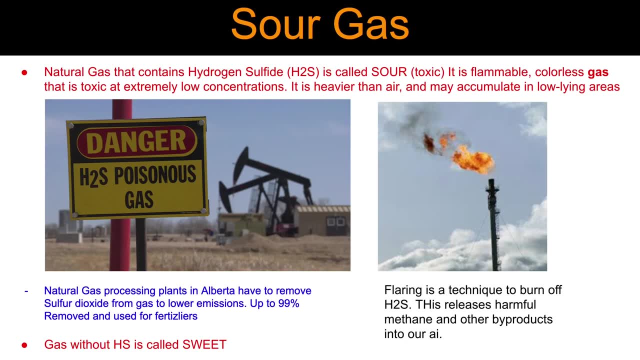 it releases CO2 gas, which we know is bad, and water, H2O, which actually isn't safe, really at well. So sour gas- natural gas that contains hydrogen sulfide- is called sour toxic. It's flammable, colorless gas is toxic and extremely low concentrations. It's heavier than air and may. 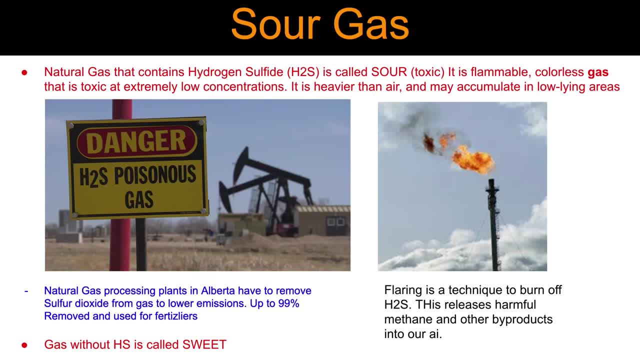 accumulate in low-lying areas. We as well have this problem with this hydrogen sulfide, because we have this natural gas and a ton of it, and so there's going to be these signs that you're looking at right now: danger, lots of poisonous gas, So you don't want to be around there breathing. 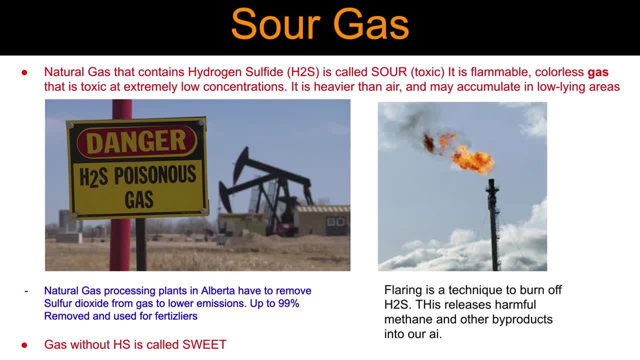 that in Natural gas producing plants in Alberta have to remove sulfur dioxide gas to lower emissions- up to 99 percent removed- and use it for fertilizers. Here's a flaring technique used to burn off that gas. You might have seen this before. You might have driven. 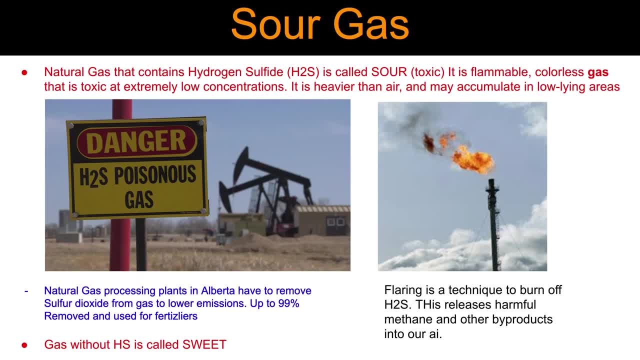 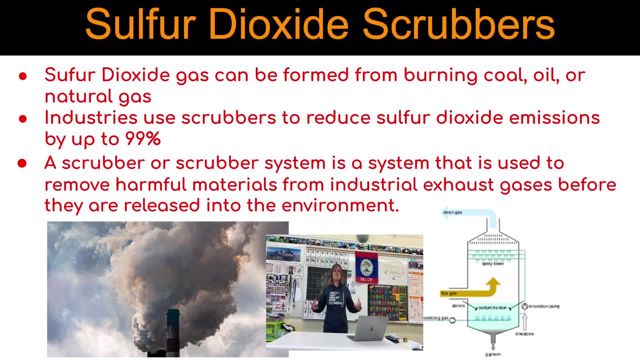 by this sort of stuff. when you see like the flames burning, They're really just getting rid of harmful gases. Gas without hydrogen sulfide is called sweet gas. I want to talk a little bit about scrubbers, and this is basically the end of this lesson. Scrubbers are actually things on the very 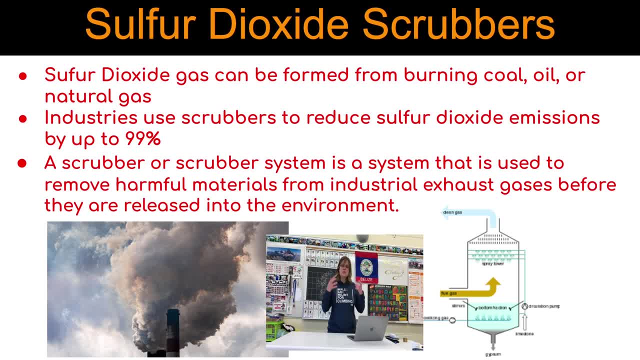 top of your industry pipes that release smoke into the atmosphere. Sulfur dioxide- anything dioxide- is bad in the environment. So if you ever see any dioxide- and I'm asking you a question- what's a bad gas? Anything oxide is bad: Sulfur dioxide, nitrogen dioxide, carbon dioxide. 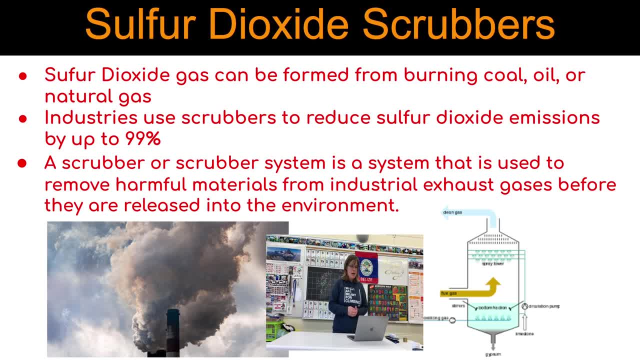 bad, bad, bad, bad. Anything. dioxide is just bad, okay, And so sulfur dioxide can be formed from burning coal and oil, which obviously we do in Alberta. So industries have to use scrubbers- That's what we call them. This kind of sounds funny, but they actually put this little piece. 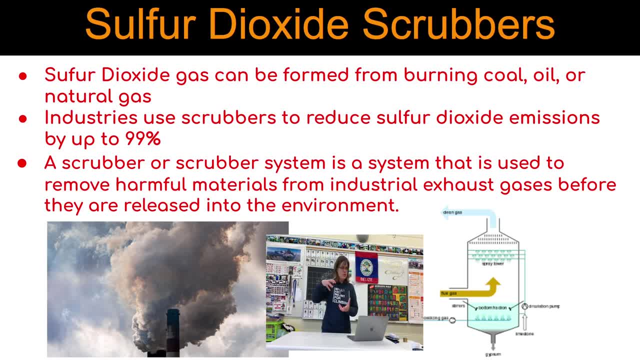 on the very top of their nice little pipeline and a scrubber is a system that uses and removes the harmful materials inside of the gas before it releases it into the environment out of the gas. So when you drive by all those pipelines and you think